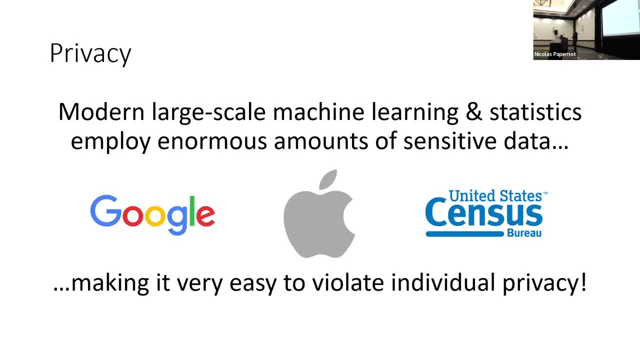 motivate privacy too much to this audience. you know secure and trustworthy ML, but I'll give a few examples more to illustrate the style of disclosure that we want to prevent. and let's start with this xkcd comic, which we'll see in many talks on privacy. You can see what happened. 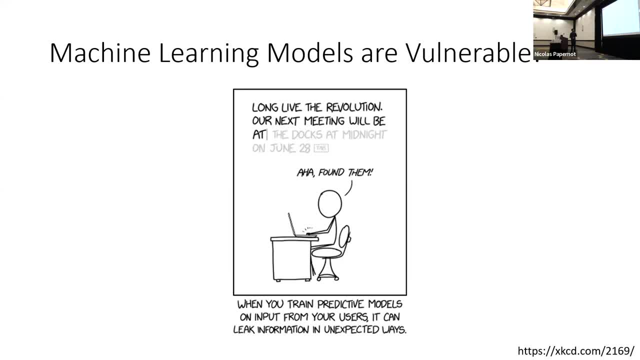 here is an individual is at their computer. They typed into their email client let's say: long live the revolution our next meeting will be at. and then they ask the machine learning system in their email. So they sent us a message and it says the machine learning system is at the docks at midnight on. 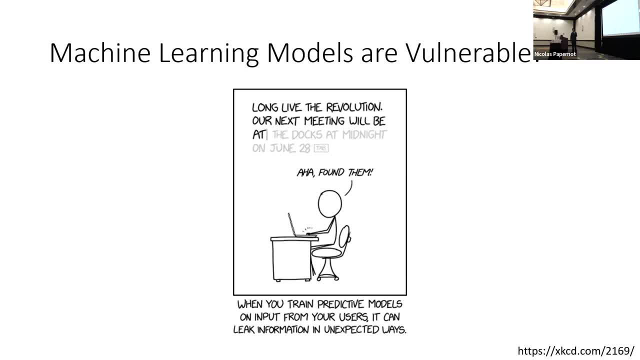 june 28th, And the joke here is, you know, as the caption says, essentially it suggested someone else's secret as the completion to their email that someone else is going to be doing something potentially illicit at the docks at midnight on june 28th, and now their secret has been leaked. 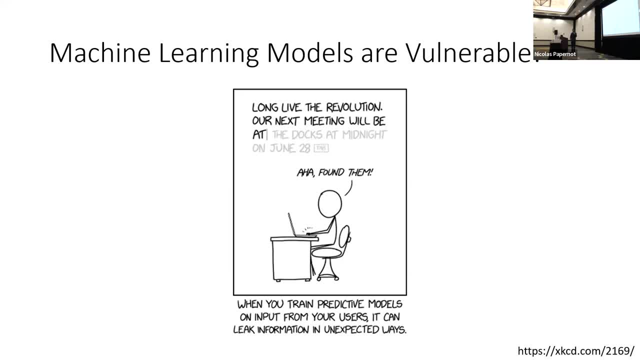 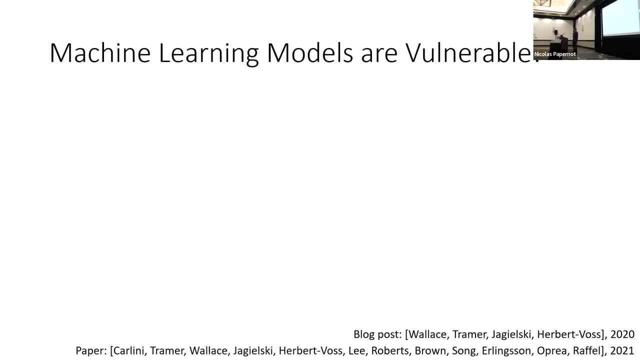 So that's a joke, it's just like a comic. so you know this isn't real, but reality resembles comedy sometimes, and there's a very nice work by Carlini et al, which I'm going to use to illustrate this, which demonstrates that machine learning models can leak information about their training data, which is problematic. 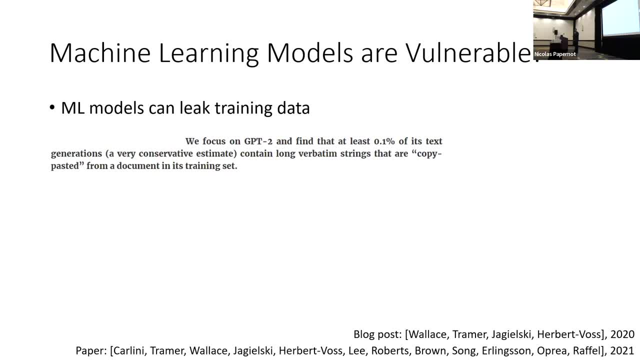 when this is sensitive. So here is from this blog post by some of the authors and they find that GPT-2 essentially copy-pastes a large fraction of its text generations from the training data. 0.1 is a fairly large fraction if your training data can be considered sensitive. 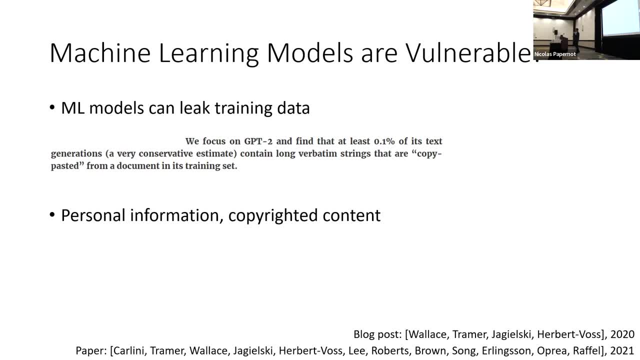 It can be here, because you'll see that GPT-2 is trained on a bunch of stuff which includes personal information, copyrighted content and more. As one illustration from their paper here: if you prompt GPT-2 with the right prefix, it'll give you out someone's personal information. 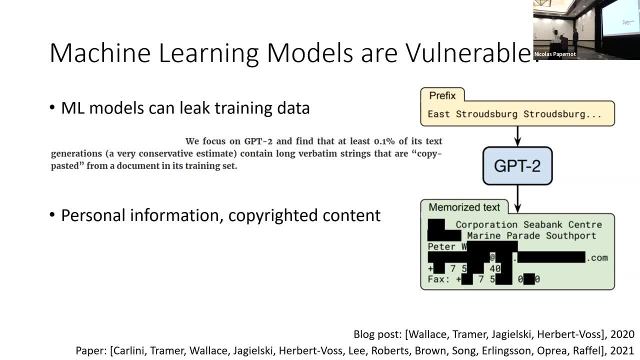 which here, for the purposes of their paper they redacted. But if you feed it into GPT-2, then it won't redact it for you. It'll tell you their name, email contact information, fax number, etc. 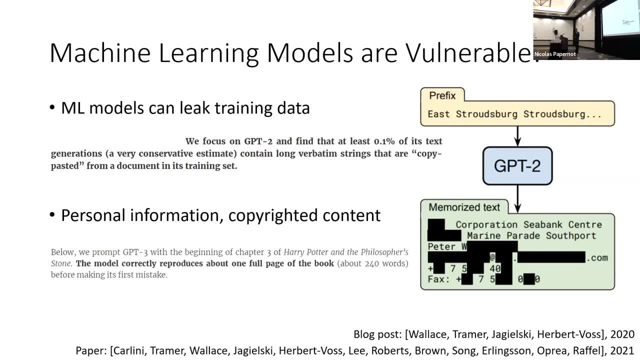 And then there's more They also find in this blog post. they mentioned that GPT-3, it can. if you prompt it the right way, then it'll spit out an entire page of Harry Potter and the Philosopher's Stone, which clearly has some important copyright implications. 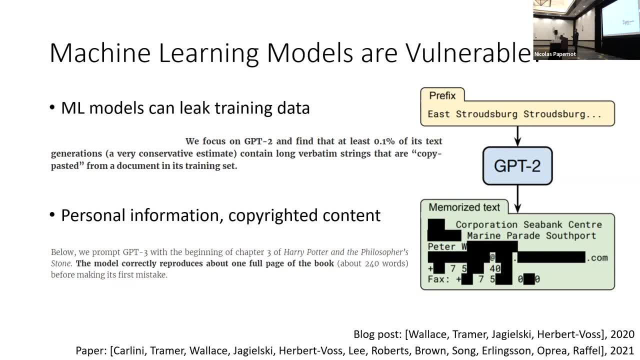 So you might be thinking: okay, these are these massive machine learning models which are very complex and they can maybe memorize their data because they have so many parameters and stuff like that, But at the other end of the spectrum, for even more basic things as well. 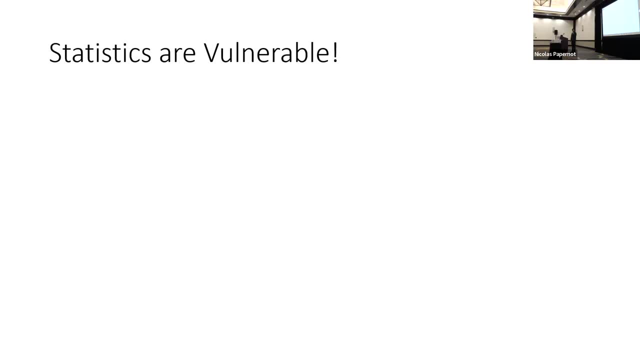 even basic statistics are vulnerable, So I'm not an expert on biology-related things, but there's something that people do, which is known as a GWAS study, which tries to find correlations, essentially between diseases and genetic markers known as SNPs, as they're called. 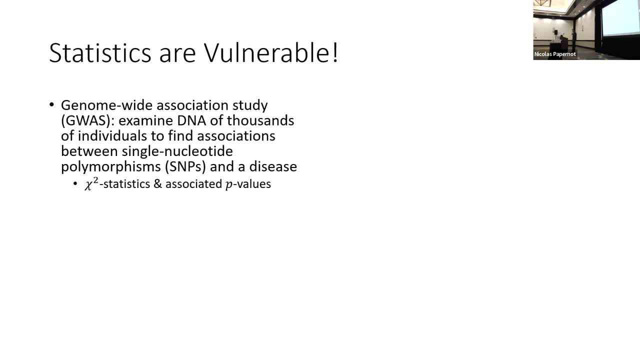 And these are computed via various chi-squared statistics, associated p-values, very simple statistics. And this is a picture of what Google Images tells me the GWAS study looks like. You can see correlations between the time of the first step of the study with the first step of the study. 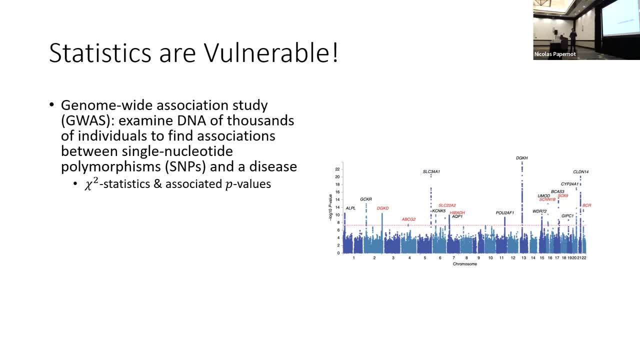 between various chromosomes and- uh, uh yeah, various different uh diseases. i guess these are so naturally, i don't have to tell you that when you're doing this sort of g-watt study, this is highly sensitive medical data. for example, you may have people participating in certain medical 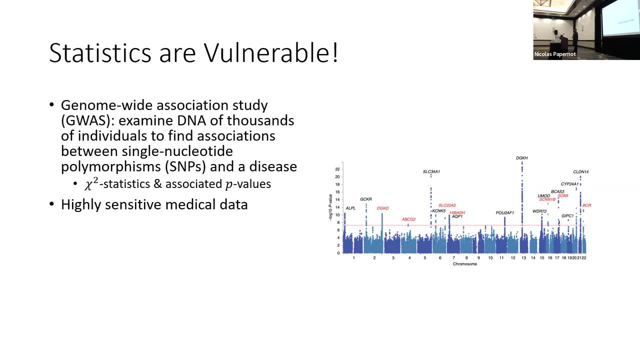 trials which are for socially stigmatic diseases, and they agree to participate in this, but they might not want the fact that they participate to be revealed because, uh, for example, something which is socially stigmatic like hiv aids, then maybe they wouldn't want their positive status to be. 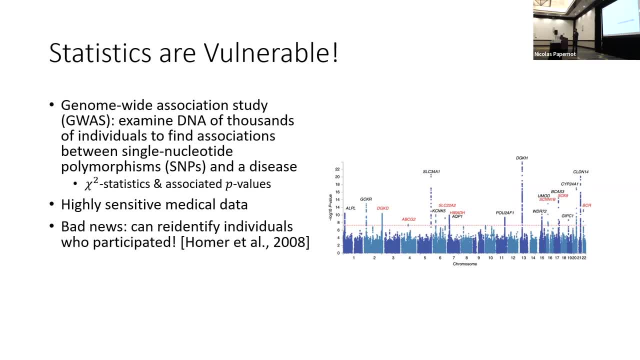 revealed, unfortunately. there's a very nice work by homer et al in 2008 which said: under certain conditions, you essentially can identify who participated in such a study, uh, which has very significant privacy implications- uh, this is known as a membership inference attack: uh, to be able to infer whether someone was a member of the uh data set which was used to do one of 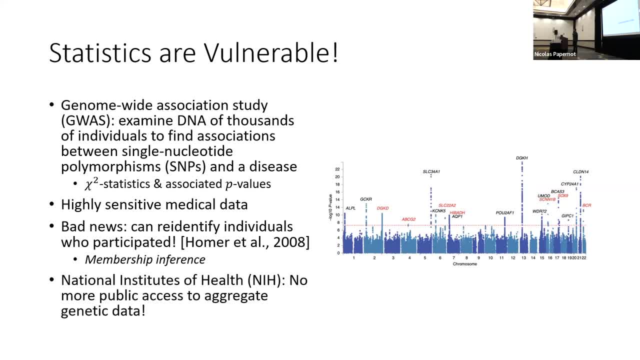 things like this. and then they were able to identify who participated in such a study. and then they were able to identify who participated in such a study, and so this was taken very, very seriously. for example, the us national institutes of health uh, essentially said, okay, this is a big. 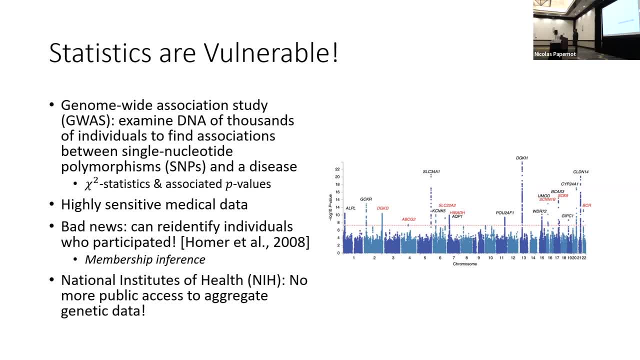 problem. we're not going to give public access to a bunch of aggregates about genetic data, and now if you want to be able to use this- uh, scientific data, you need to go through a lengthy approval process. so this seems like a pro problem and we would like some way to do this sort of data. 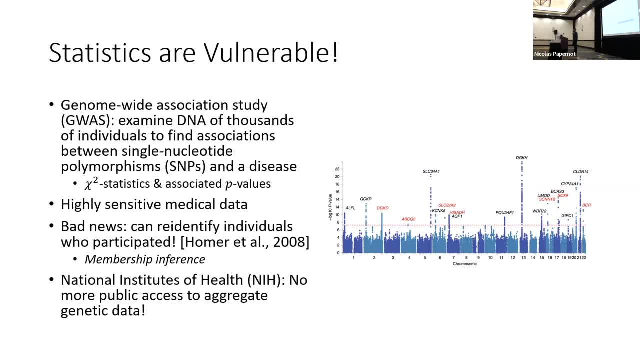 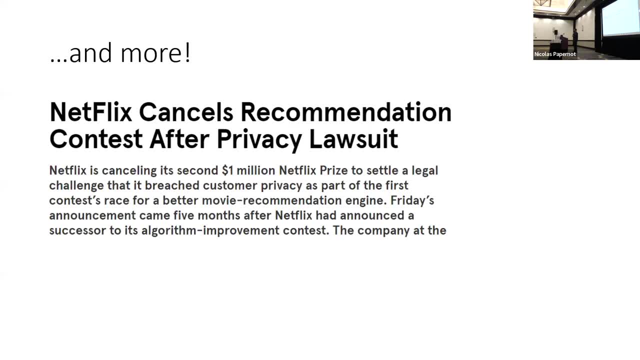 analysis while respecting the privacy of the individuals who gave their data. and these are just two examples. there's many more. i could give another hour-long talk, just telling you all of these. for example, there's a netflix prize. there was a major lawsuit against netflix because they didn't properly anonymize the data set. uh, i think this title tells you. 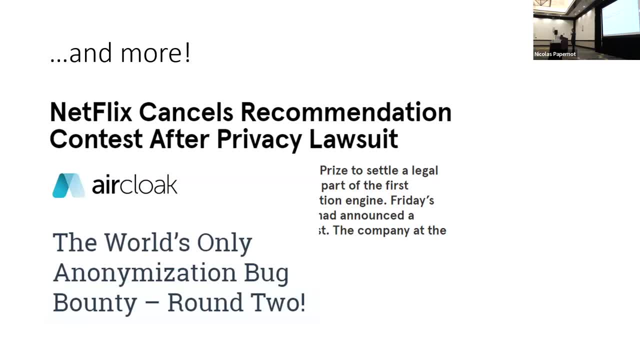 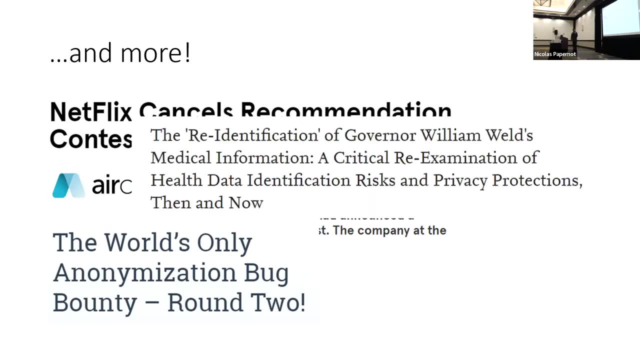 everything you need to know. round two of an anonymization bug bounty, um, this was this is about. round two is also quickly broken as well. uh, there was the mass gic incident, where the governor of massachusetts will weld was mailed his own medical documents due to inability to anonymize. 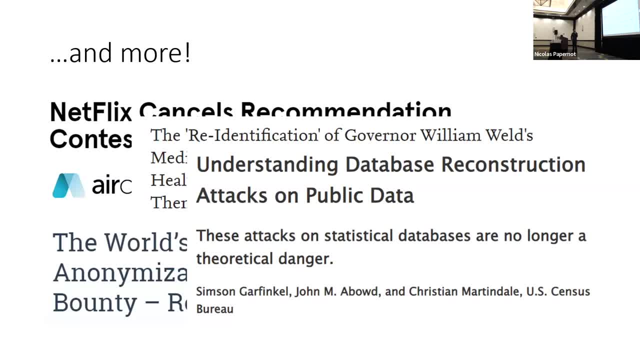 data appropriately. and, uh, notably one recent application has been in the census where, uh, some census researchers essentially attacked the census and found they could attack the census and re-identify certain individuals. so the common trend here in all these cases is, it seems like large-scale ml. 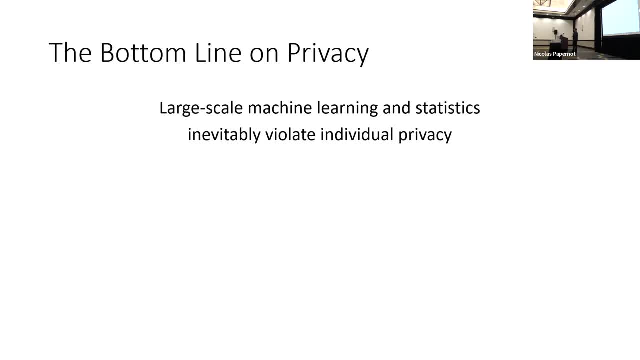 and statistics will inevitably violate individual privacy of the individuals who provided their data for the training data set and we've seen time and time again- people still have a tough time believing this- who don't work in privacy. but best effort or heuristic privacy won't and don't work um aggregation only reporting, aggregate statistics, things like anonymization. i 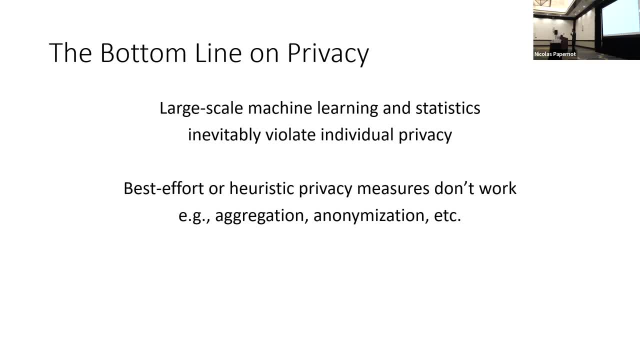 think there's a great quote attributed to cynthia dwork which says: anonymized data isn't uh, and you know, really, i think this motivates that we need rigorous privacy guarantees in order to preserve user trust if we really want to do uh, private and reliable machine learning, so that 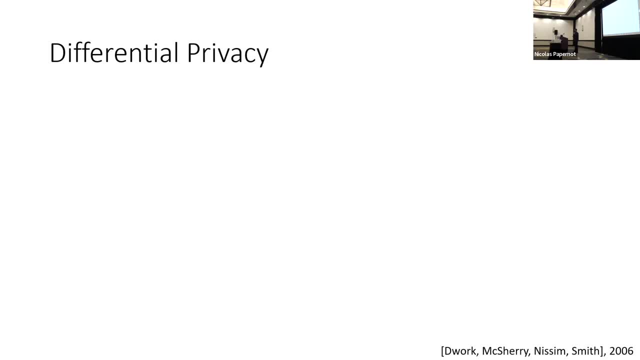 brings us to the uh definition, or the definition of differential privacy, which was introduced by smith in a very influential paper in tcc 2006.. um yeah, i'm going to first sort of it's differential privacy, the first. like five, ten times i saw the definition i was like okay, this is a. 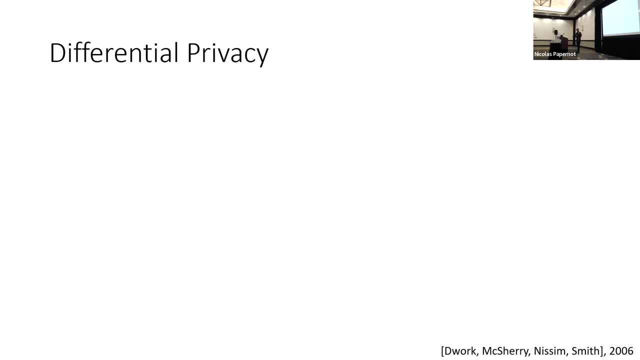 little bit, uh, tricky. i don't know what's going on here, so i'm going to give you first this kind of illustration about how i like to think of privacy, or maybe how you should think about privacy. then we'll see the definition and discuss it. uh, please, don't you know if you, if you find the definition. 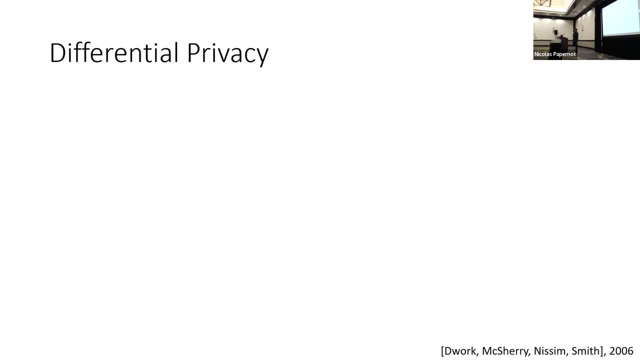 a little bit intimidating, don't worry, you don't need to like understand all the intricacies again. that would take several hours to really really understand why everything is the way it is. so, um, yeah, don't be too intimidated when you see it. but again, to illustrate at a high level how i like to think of differential privacy and what 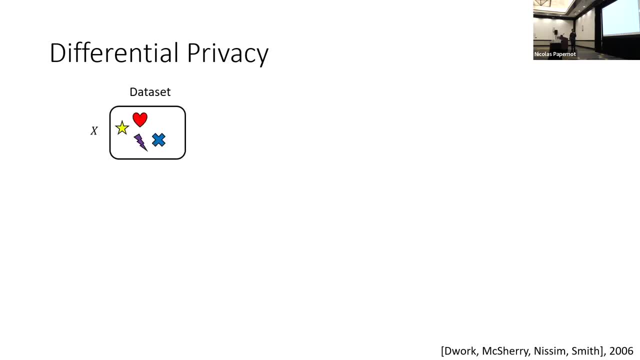 it's trying to protect. imagine the following type of scenario: we have some data set x which is fed into an algorithm and it produces an output. now we could imagine, alternatively, a data set x prime, which is similar to x but it differs in, say, one entry. one entry has been added, let's say it instead- could be fed. 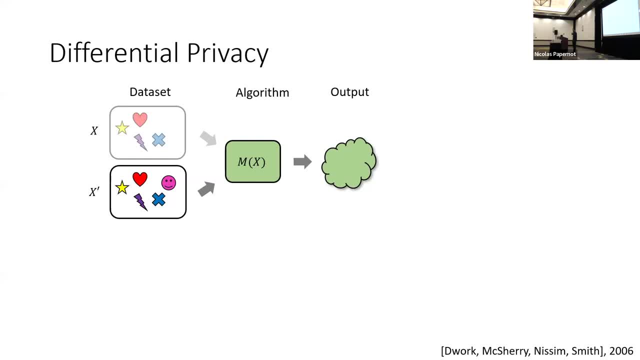 into x or m of x the algorithm and produce an output. now the idea is, an adversary is going to be looking at the output of this algorithm and what they're trying to do is they're trying to figure out which one was fed into the algorithm with an x or x prime, and if the adversary is 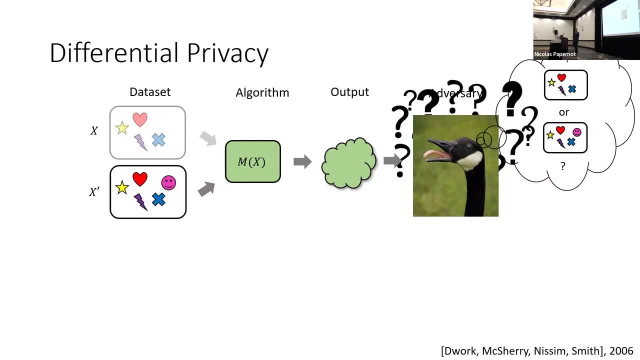 unable to really figure out or ascertain which of the input data sets with x or x prime. better than, say, random guessing, maybe with a little bit of advantage over random guessing. then we say the algorithm that produces output is differentially private. so this is like a little bit of an. 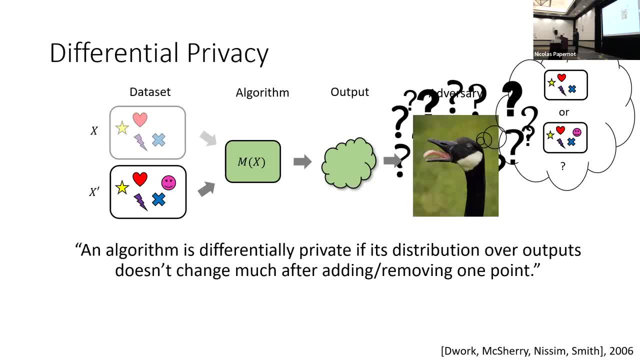 informal explanation on how i like to think about it, and again in words. we say: an algorithm is differentially private if it's distribution over outputs doesn't change much after you added or removed one data point to the input data set. so let's, let's. that's a very odd and specific. 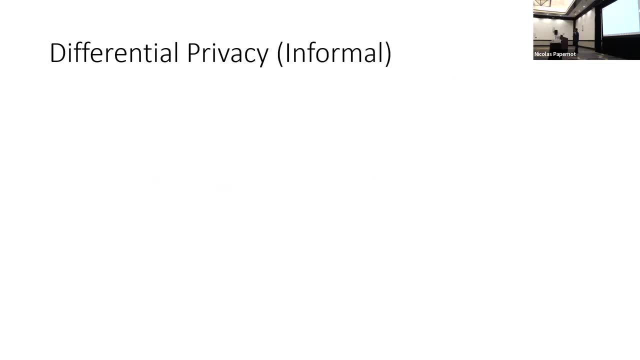 definition, uh, informal definition. let's let's investigate a little bit. why does that uh imply any sort of privacy set for the training, data set to individuals? and i'm going to walk you through an informal argument which is formalizable in some way, but just to sort of convince you that this is reasonable. 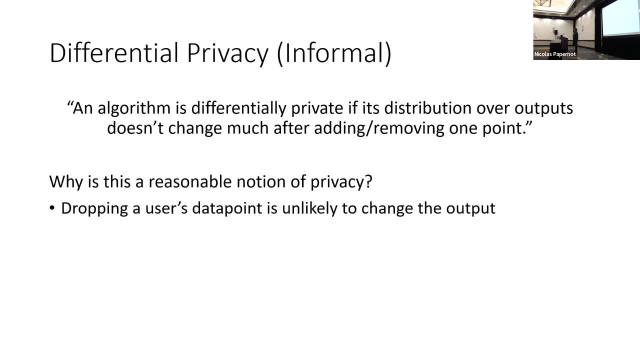 based on this informal definition, dropping a user's data point is unlikely to change the input. just that's exactly what it says. the distribution won't change too much. therefore, if you look at the output, you can't really tell whether a user within the data set or not. and that's even in the very strong case where you know exactly what that user's data was. 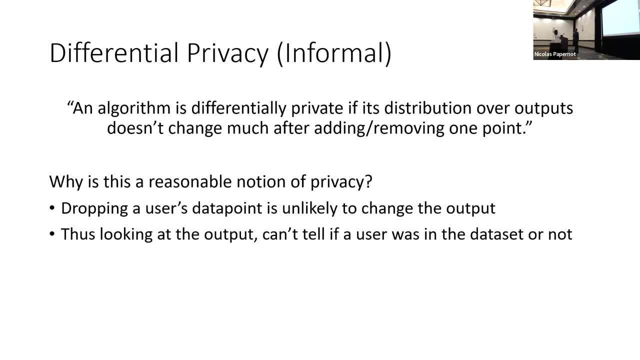 you can't fix it, you can't figure out whether they were in the data set or not. that's a very strong guarantee. if you can't even figure out whether an individual was in the data set or not, then there's no way you can even guess anything about, uh, what their data point actually was, and so that's, that's kind. 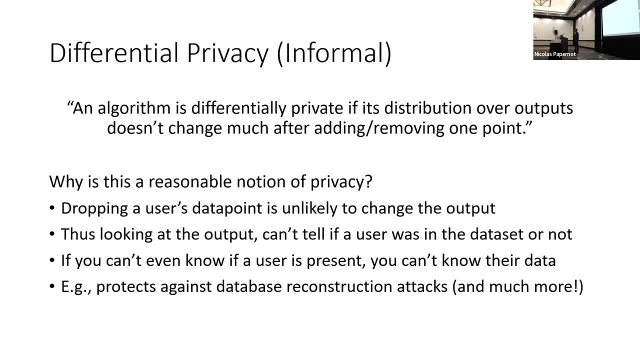 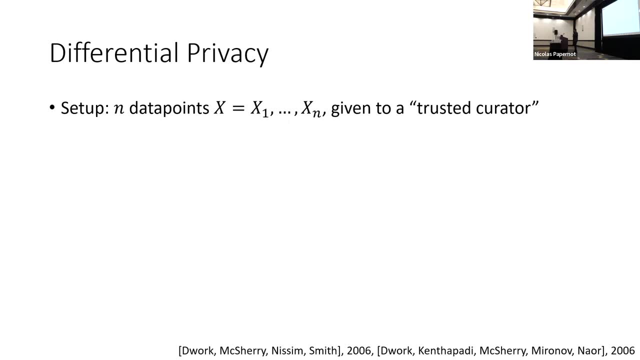 of informally, why, uh, it can prevent a lot of types of attacks, including a lot of things which i'll i'll give you a few examples, uh, a bit later. but, in particular, everything we've talked about so far is prevented using differential privacy. cool, so this is now where i'm going to introduce the actual definition. again, it's a bit 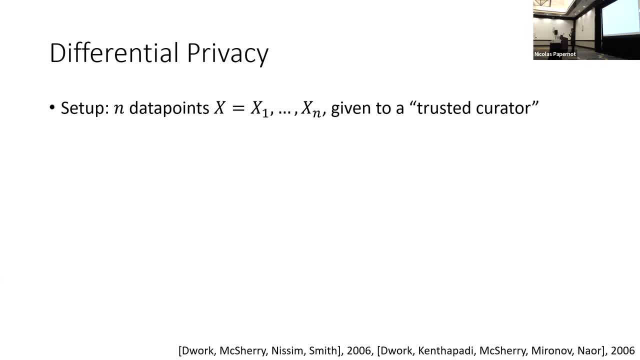 intimidating at first. i'm going to introduce it. we're going to discuss it a bit, but if it still goes over your head, don't sweat it. we can make it through the rest of this talk. we're not going to rely on it too heavily, but the setup is the following: we're given a data set of n data. 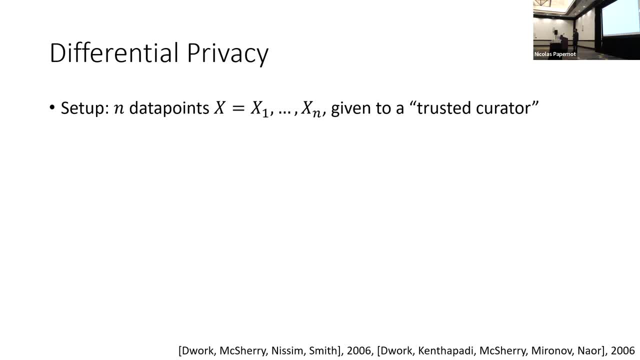 points which are sensitive in some way, and these are given to what's known as a trusted curator. a trusted curator is someone who you trust in two ways: one, that it's okay that they see the data and manage the data, even if it's sensitive. and two, you trust them that, uh, they won't report. 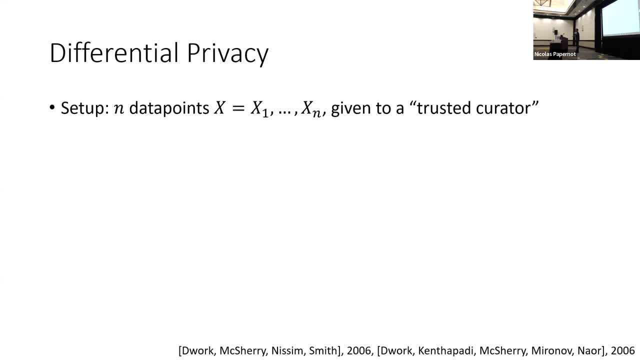 anything which is not differentially private. so this might seem like a strong assumption like why would you trust anyone with your secret data? but for a canonical example, say for the us census, you trust maybe the us census to accept your sensitive data, but you know and trust them not to just put this data out on the internet publicly for everyone. and 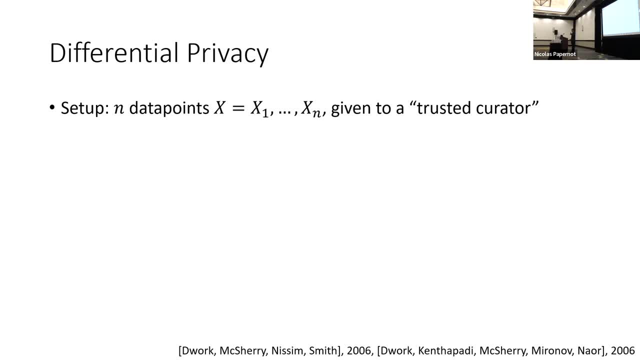 do responsible things. there are other models where you can look at, where there's no trusted curator model, but we're not going to get into that today. but it can be more realistic in some settings. but yeah, we're going to look at the trusted curator model and we're going to say: the curator. 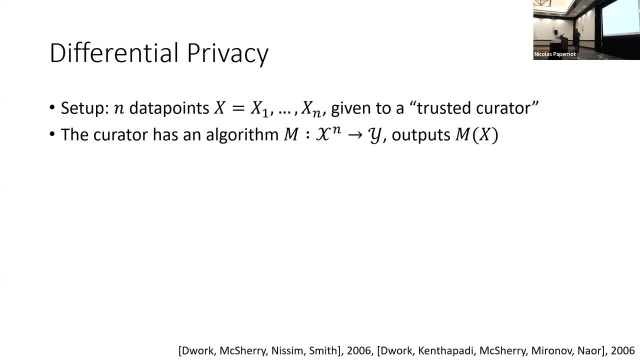 they essentially have an algorithm that takes in some data set which is of the appropriate type and uh. it outputs something in the range space y, uh, and yeah, they're going to output whatever this algorithm gives on the uh data set which is sensitive. so this is the definition which, again. 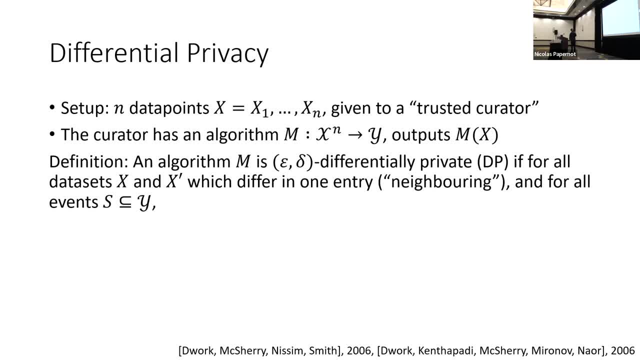 is a bit of a mouthful. um, there's something missing still, but we'll get to it. um, we say that an algorithm is epsilon, delta, differentially private, or dp for short, if for all data sets x and x, prime, which differ in one entry, that's neighboring. uh, you, i showed the picture before. 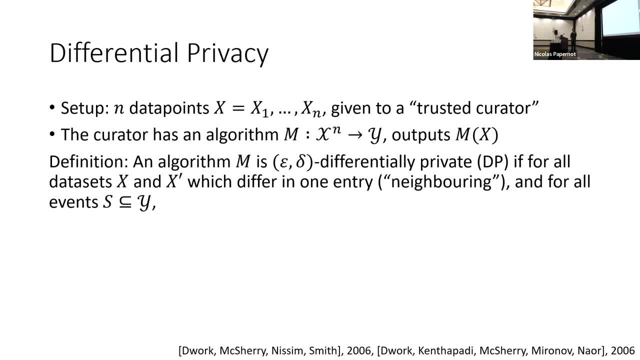 where you add or remove one data point and for all events uh, which are subsets of the range of this algorithm, we have the following uh guarantee: again, this is a little bit uh intimidating at first, so don't sweat it. if this uh doesn't make full sense, we'll discuss it a little bit more. 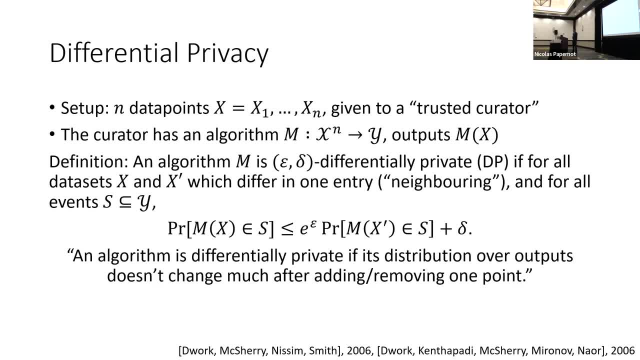 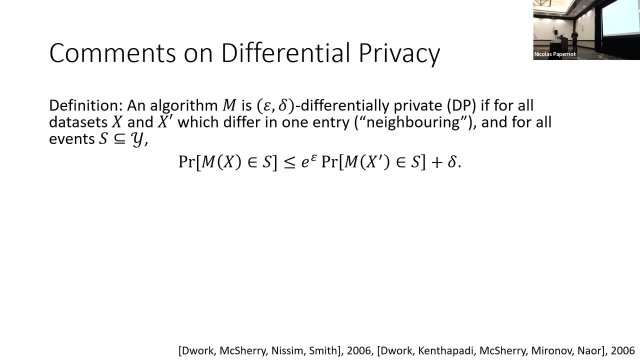 you, uh, and you know, again, keep in mind the intuition which i gave there, which is how i would describe this in words: uh, the algorithm's distribution over outputs that it can give doesn't change much if you add or remove one data point. cool. so let's, let's investigate this definition a little bit more and, uh, look at some of the. 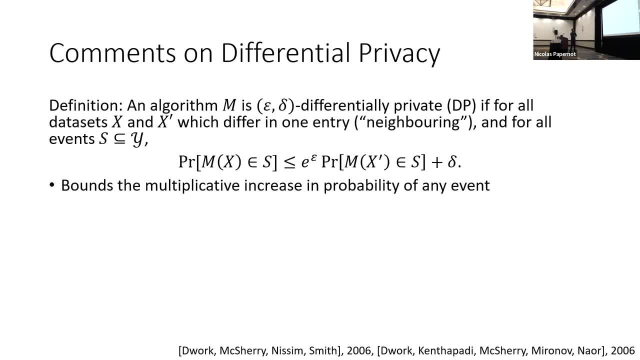 salient features of it. so the first thing you can see is: let's, let's ignore delta, pretend delta doesn't exist, it's zero for now. first of all, you'll see that it kind of bounds the multiplicative increase in value of the data set. so let's look at the salient features of it. so the first thing, 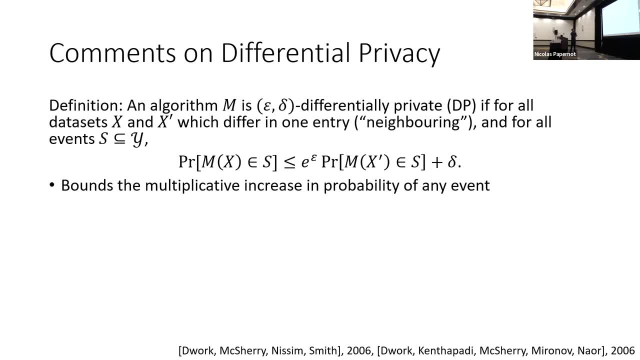 is the probability of any event like this is the probability that uh s happens on data set X and this is the probability that s happens on uh data set X prime, and you can see that there's this multiplicative bound on how much more likely it can be. it's not going to be a million times more. 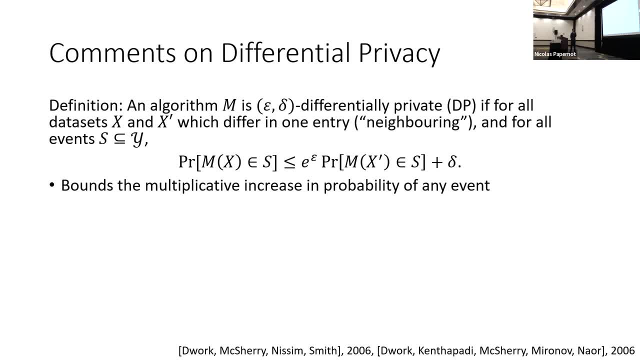 likely, it's going to be e to the Epsilon times more likely, which is fairly small. if Epsilon is, say, small and uh, there's a small additive change which is permitted as well. but basically you should mostly think of it as this multiplicative increase in the probabilities. 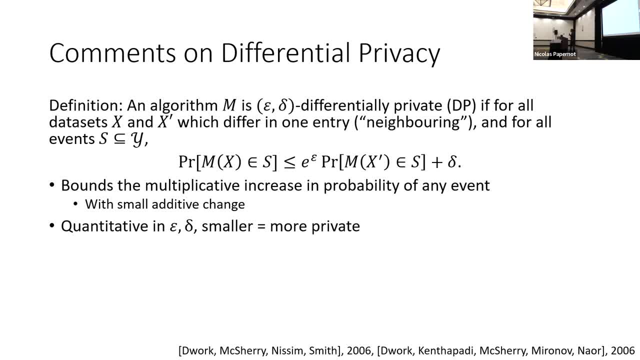 the. the most important and one of the most useful things here is: this is a quantitative definition, in the sense that you can have stronger privacy if you set Epsilon and Delta to be smaller and it's weaker privacy if Epsilon and Delta are larger. so say Epsilon and Delta equals zero. 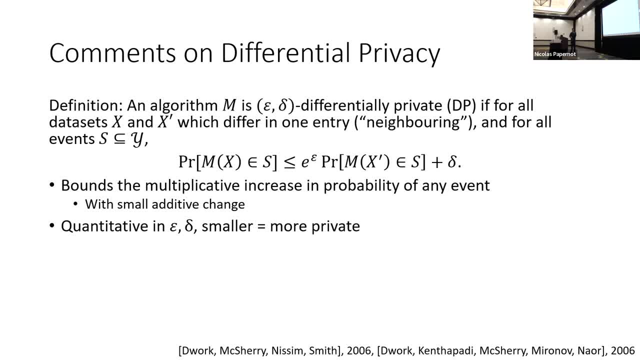 you can sub it in there, that'll just ignore the data set. if you set Epsilon and Delta to be, say, Infinity, then you'll see that, uh, this, this captures any algorithm. there's no, and any algorithm you've run is Infinity, comma, Infinity, differentially private, for example. 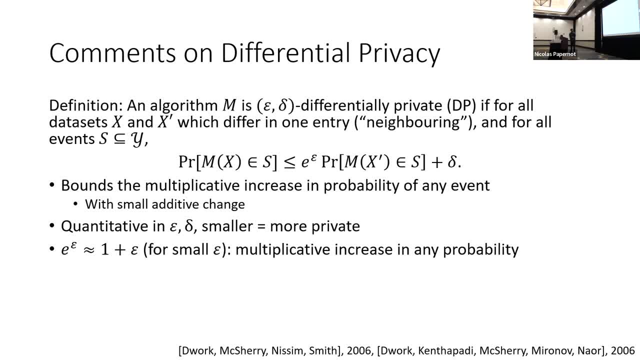 and to give you an idea of how these two play in. so let's, let's look into the quantitativeness of this. so you see, this e to the Epsilon. it's a little bit odd, but for small Epsilon you can think of that as roughly- uh, you know one plus Epsilon if you have a. so it's a small multiplicative. 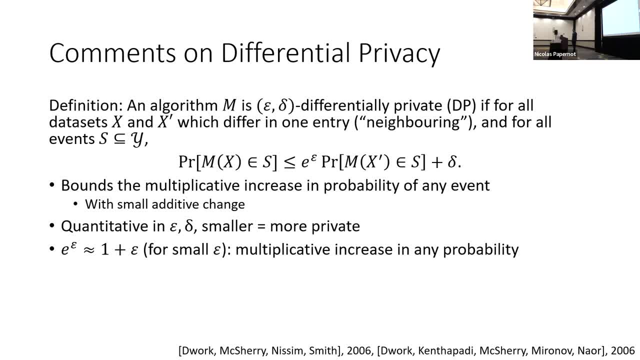 increase if you have a small Epsilon, and that's how much the probability of any event can increase. keep an often. people often ask: how big should Epsilon be? uh, the rule of thumb something in the neighborhood of around one is reasonable. uh, sometimes you'll see smaller sometimes. 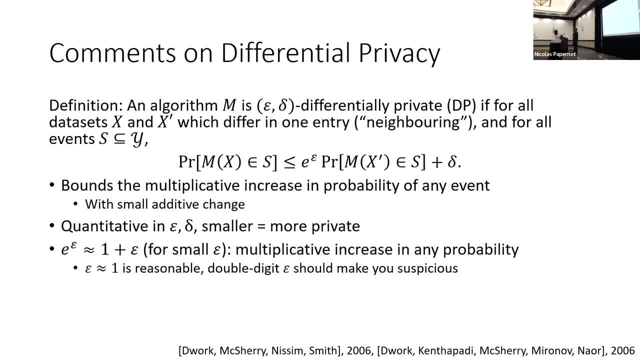 you'll see larger. I think the alarm bells in your head should go off if you see something greater than 10, because E to the 10 is a huge number, but even sometimes things as large as eight can give reasonable privacy guarantees. we can discuss that a bit more offline, but roughly, you should think. 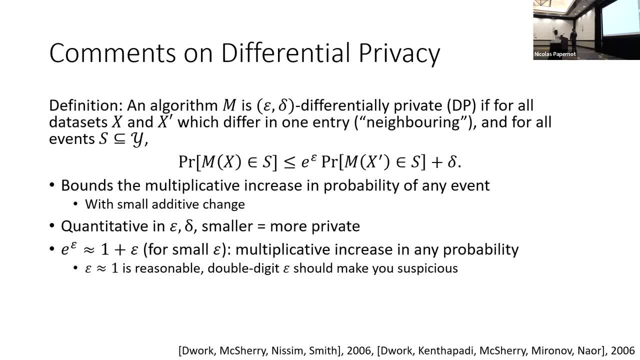 maybe one, two, three. that's pretty strong privacy. uh, Delta you can think of as, in some informal sense, the probability of a potential total privacy failure, like, for example: think with probability Delta, we just give up and output the entire training data set. some massive privacy violation, uh, is what could happen. so, as a consequence, this Delta, we typically want it to be rather small. 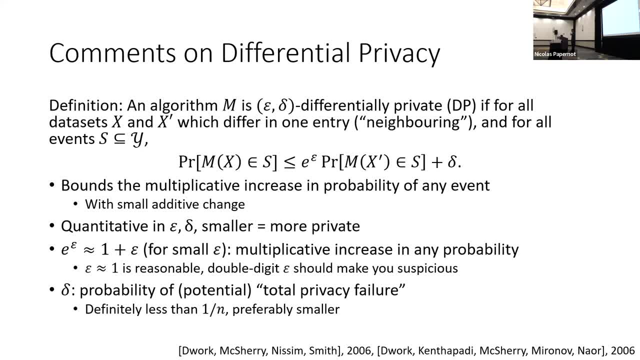 like at most one over n, where n is the data set size, but preferably smaller. so good, this is a lot of discussion here, but roughly speaking, you should take away from this slide that it's a quantitative notion of privacy which depends on Epsilon and Delta, and smaller equals more private. 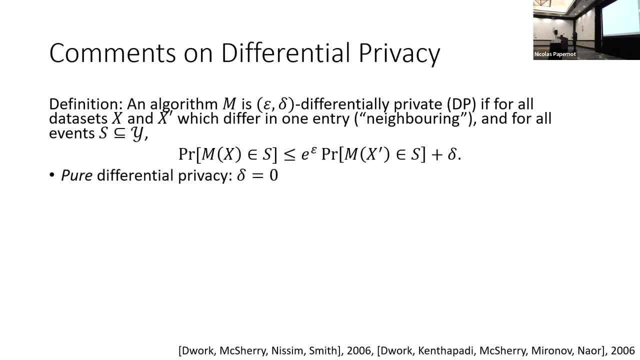 uh, there's a bit more discussion. I want to get here in the sense that there's two, there's many kinds of differential privacy, you've heard. uh, maybe the number of important ones in my opinion is about like on the order of five different notions, but today we're going to be focusing on sort of the. 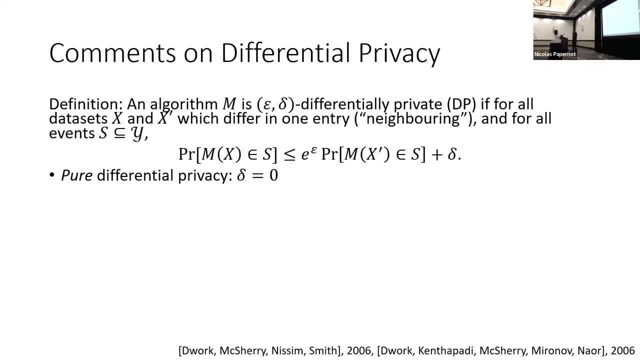 OG ones. uh, pure and approximate differential privacy here. differential privacy is when Delta equals zero. uh, this is kind of the one that was defined in the original Dwork at all paper, uh, but then the Delta that was introduced in another Dwork at all paper in the same year, but that's. 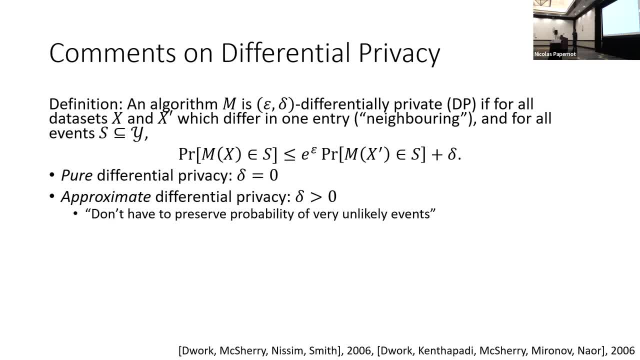 often called approximate differential privacy and the. the intuition here is it can sometimes be very, very hard to preserve the probability of absolutely every event, in the sense that the original definition of pure differential privacy, even if you have an event which happens with probability- uh, you know- 10 to the minus 100 or something you still have- 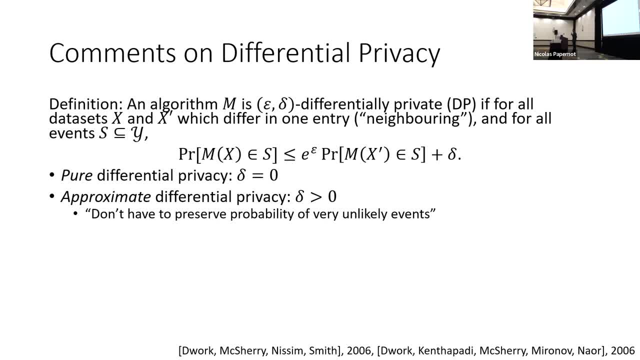 to have this very strong guarantee that that somehow you have to preserve the probability of that event. so this, this, that can be a bit restrictive sometimes, and this Delta was introduced to allow basically- maybe roughly speaking, you think, uh- events with probability of much less than Delta. you don't really have to worry about those and uh, you know they're, they're. 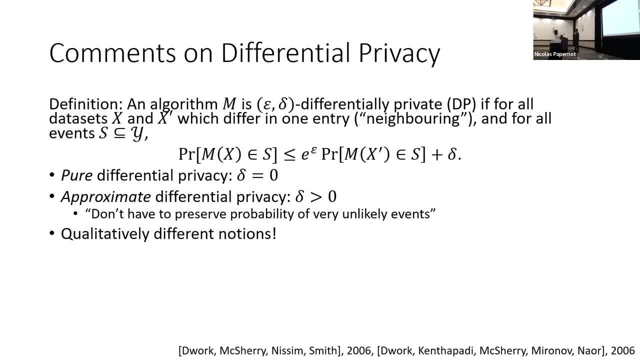 not really things you have to worry about with privacy- and these turn out to be qualitatively different notions, in the sense that there's some algorithms which work for approximate DP which don't work for pure DP. um yeah, we'll talk a bit more about, uh, when to use different definitions. 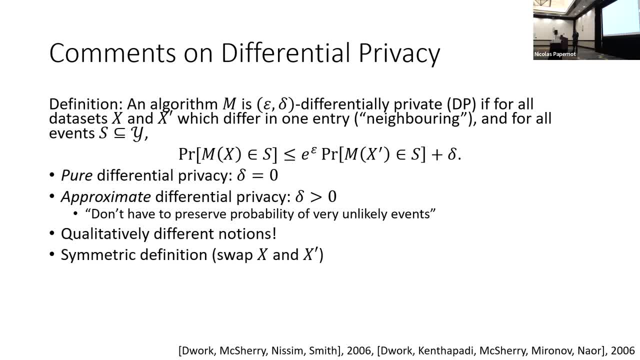 a bit later. uh, a few more, just minor notes. one is that this is a symmetric definition. you might be wondering: why is there an upper bound but no lower bound? if you just swap the location, it's an x prime. effectively you have the lower bound as well. but this is a more succinct and 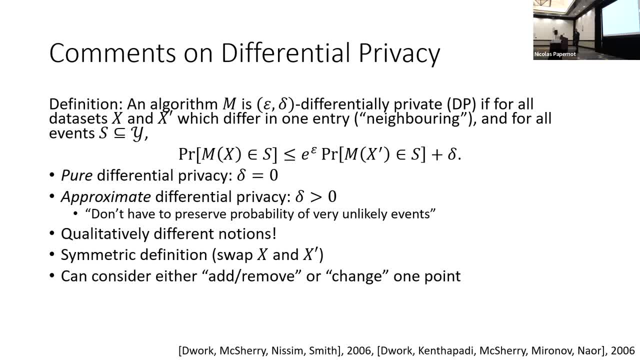 common way to see it. um, and finally, I've talked about- you know, I've sort of muddled my terms in terms of, uh, adding or removing a point versus changing a point, uh, you'll see both definitions and in very rare cases makes a difference, but, roughly speaking, the idea of adding, removing, 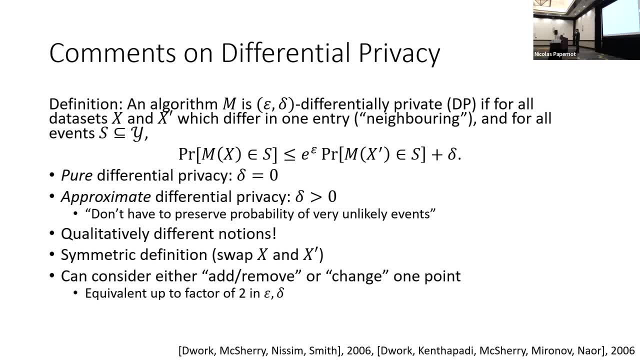 changing a point or equivalent up to a factor of two. uh, where? so don't don't worry too much about that specific detail for the purposes of this tutorial. cool. so that's everything I want to say about, uh, the definition itself. again, it's a little bit of. 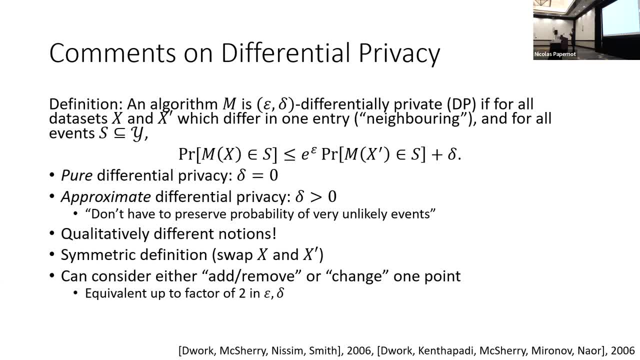 a mouthful just, but think of it again as preserving the probability distribution over outputs in some very specific and precise way that you know. we could discuss for several hours about why this is exactly the right way and why many other ways are not good enough. so let's, what can you do with? 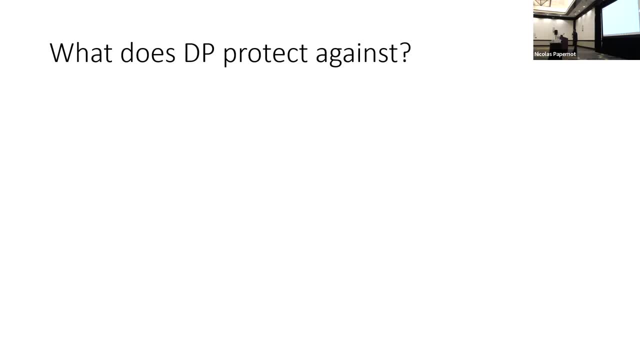 differential privacy. what does it protect against and what doesn't it protect against? um, at a high level, um, the way I like to say what it protects against is learning anything about a user that you couldn't have inferred without them, and my claim is- I'll say this again next slide. but 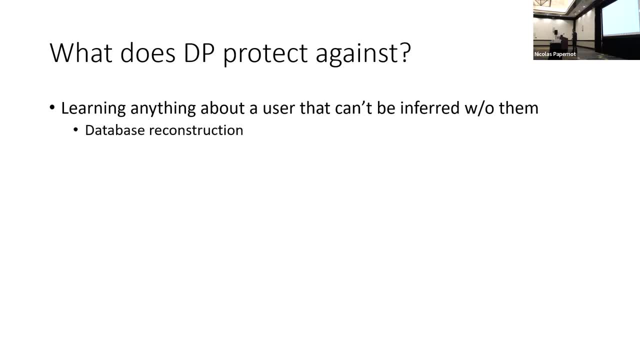 it does exactly that, nothing more and nothing less. but it protects against, for example, database reconstruction. if you have some database and it only gives differentially private answers, then, uh, that implies that, based on those answers, you won't be able to reconstruct the data set. um, it also protects against membership inference, like I mentioned before, and I don't have it on. 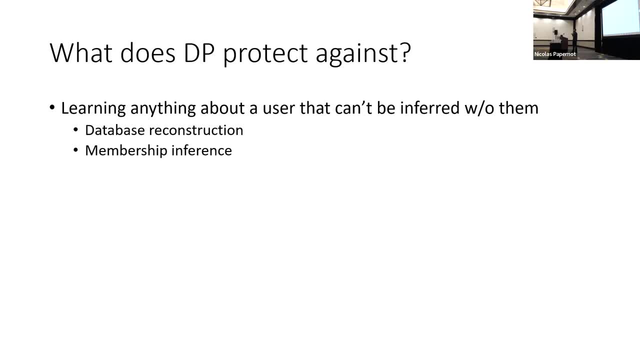 the slide, but also say that again an example of leaking your training data. as GPT-2, it protects against things like that as well, because obviously a user's individual data point is something that is sort of very bespoke to them and something that you'd protect with this definition, I think, even more important than 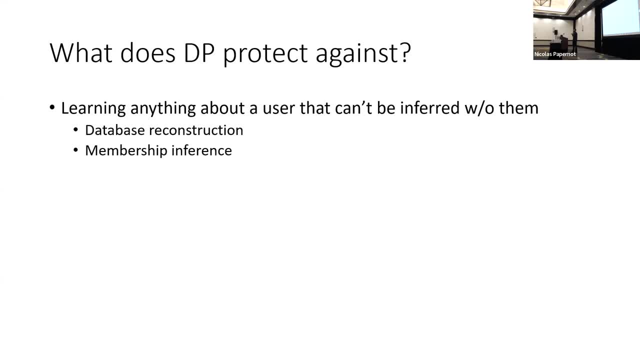 what it does protect against is what it doesn't protect against. I think this one point is the most conceptually important part of the definition which you'll see. even experts in the field of privacy sometime misunderstand this important point, which is that sometimes people claim that a privacy leakage happened, uh, but in my opinion, it didn't actually. 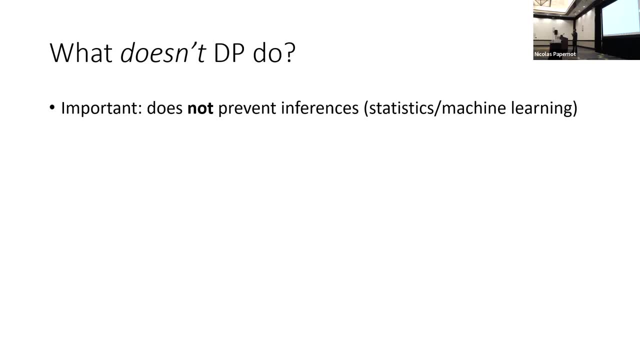 happen. in particular, differential privacy allows you to still do uh, machine learning and statistics, and that is, inferences about a population which are not specific to one individual. let me give you an example of what I mean by that. suppose someone is publicly known to be a smoker and 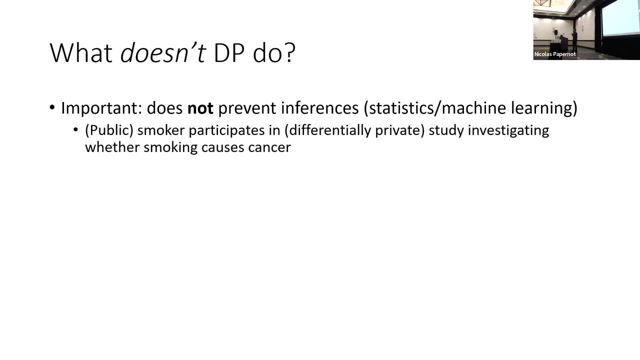 they're asked to participate in a study to investigate whether smoking causes cancer, and they're a little bit uneasy because you know what, if everyone knows that, uh, because I smoke, then I'm going to get cancer in the future and so my insurance premiums will rise. but oh, they tell me it's differentially private, so, like it doesn't matter, I'll participate in the. 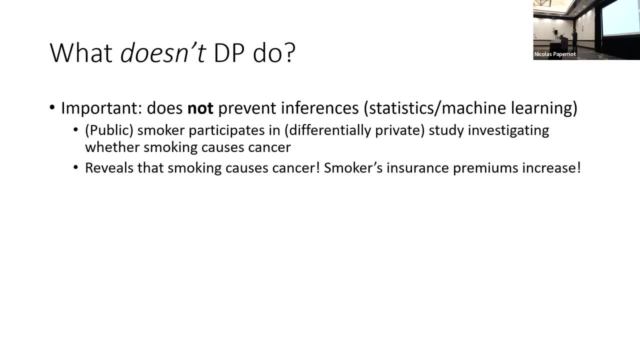 study. so they participate in the study and then it's found that smoking caused cancer. the person's insurance premiums rise. so they kind of were exactly what they had. what happened? uh, exactly what they were afraid of happened, and, you might be asking, was their differential privacy violated? 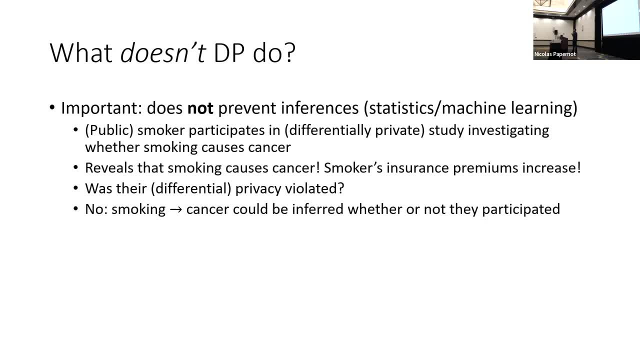 but when you think about it, no, it wasn't, because whether they participated or not, the conclusion still holds that smoking causes cancer. uh, you know, this is not their secret. it's a secret about nature that they was just discovered. so differential privacy is really about trying to. 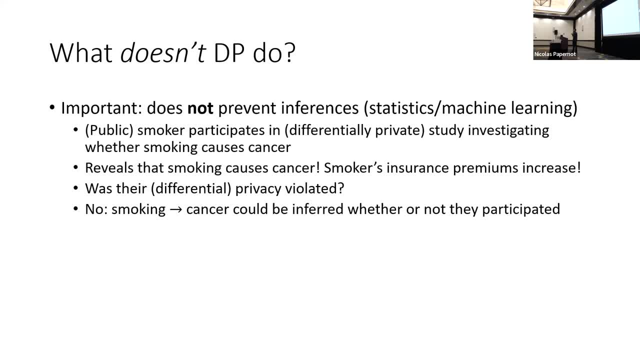 make, prevent, protect these individual secrets that are really yours to hold and keep, not things about nature itself. so that's an important distinction that uh, I think a lot of papers uh seem to miss at some points. so yeah, like I like to say, differential privacy in terms of an operational 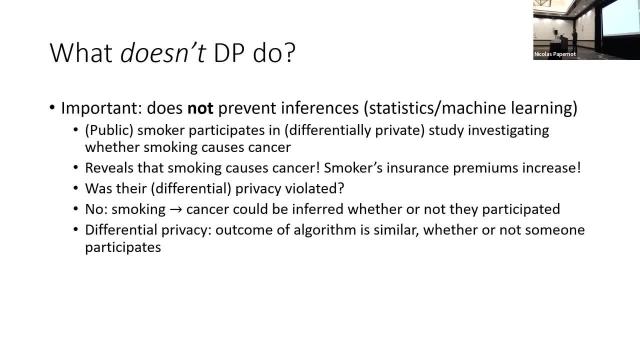 definition. it guarantees that the output of the premium is simple, similar, whether or not someone participates, nothing more and nothing less. I'll mention there's also other things which are, you'll hear, private, referred to in a lot of other settings. um, but it's not appropriate in every setting, for example. uh, one thing is: 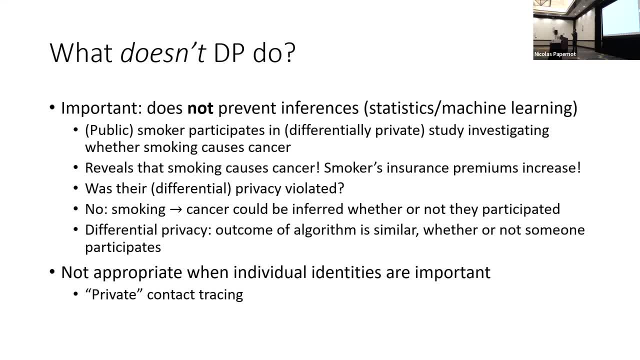 private contact tracing where you know, especially in covid, where maybe I had covid, so I need to know who else interacted with and so I can trace it back to someone. this is, you know, the word private used in a very different sense, because you really need individual. 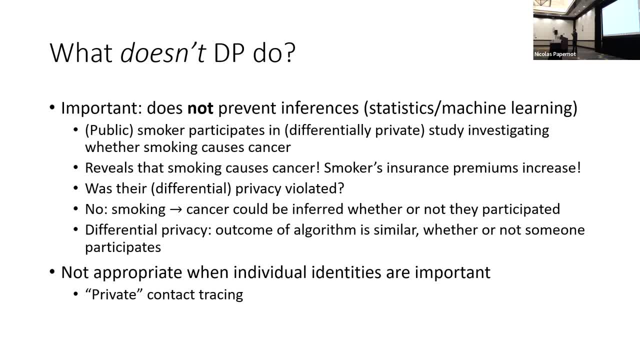 entities for this, which differential privacy really erases kind of individual data points in some sense cool. so that's the uh, that's some discussion of what it can and can't do, and it's a very popular definition for a number of reasons, uh, which I'm going to basically spend. 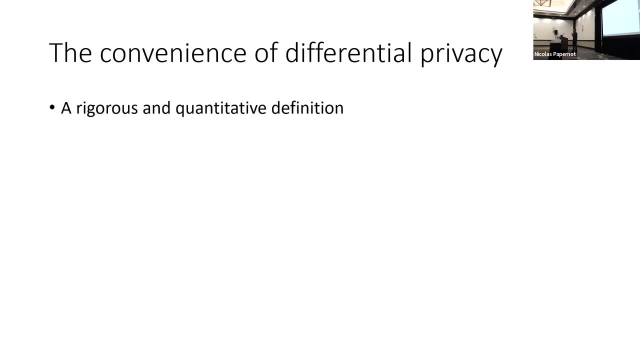 the rest of the talk going over. we've kind of already talked about the fact that this is a rigorous notion, uh, of privacy, in the sense that you prove that an algorithm is differentially private- it's not measured how private it is- you give a proof and then therefore there's like an information, theoretic fact that privacy is. 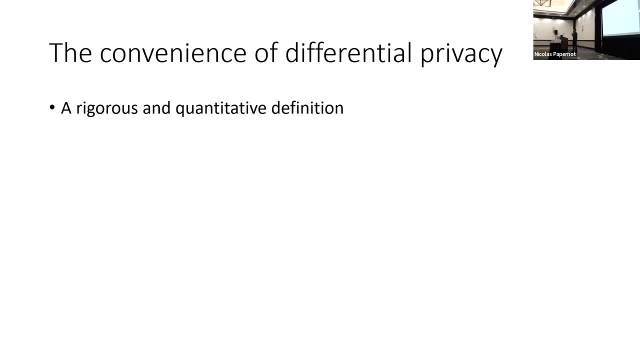 guaranteed, and it's also quantitative, which is important as well. so we've talked about this already, and the reason why it's so easy to work with differential privacy is because there's a very nice toolbox of algorithmic building blocks and machine learning tools which you can kind of 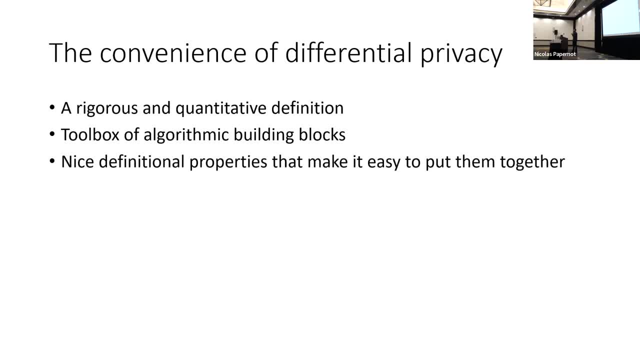 put them together in the right way, using also definitional properties of differential privacy which allow you to make you know. I'll tell you first some very, very simple algorithms which are private, and then you might be thinking: how, how could you do anything useful with that? this seems like too basic to be able to do anything. 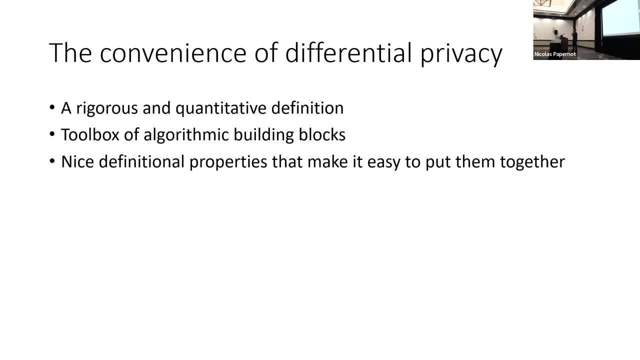 meaningful. but then I'll show you how to train an arbitrary machine learning model with even just the most basic of facts. so I think this is rather uh remarkable- how you know how you can build things which makes it incredibly convenient- so cool. the next uh segment will be focusing, like I promised. 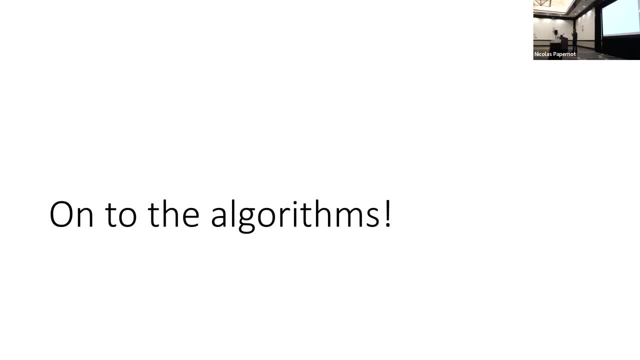 on some of the basic algorithms and tools. you know, I told you an algorithm is differentially private. uh, if an algorithm is differentially private, it means it satisfies this. but how do we come up with some actually differential private algorithms? and I'll give you two examples of differentially private algorithms. the first one is probably the 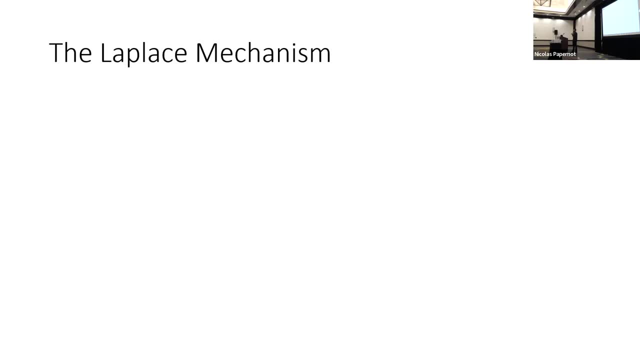 first algorithm that anyone knows when they uh start in differential privacy, known as the Laplace mechanism, I'll mention. for weird historical reasons, sometimes the term mechanism is used in place of algorithms. uh, think of them interchangeably. it's a weird term, but that's how they call them. so let's start with a very simple example. suppose our data set is x1 through. 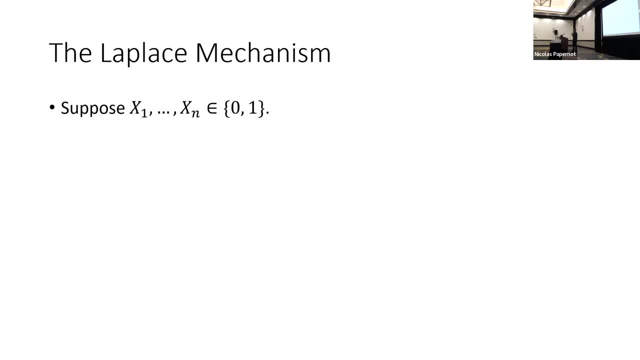 a bit zero or one, and you can think of this as, maybe, whether someone smokes or doesn't smoke, uh, and our goal is to estimate how many people in the data set smoke, and we want to do this privately, while respecting, uh, individual privacy and the notion of differential privacy that we just talked. 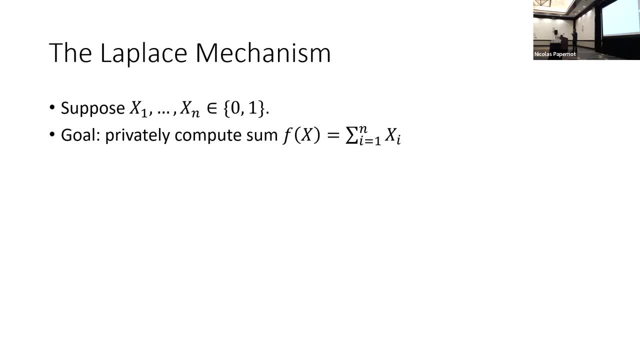 about, so how much we do this. one of the key quantities which underlies a lot of algorithms in differential privacy is what's known as the sensitivity that is, given this function that we, the function we want to privatize, which here is just the sum of the bits- how much can it change? 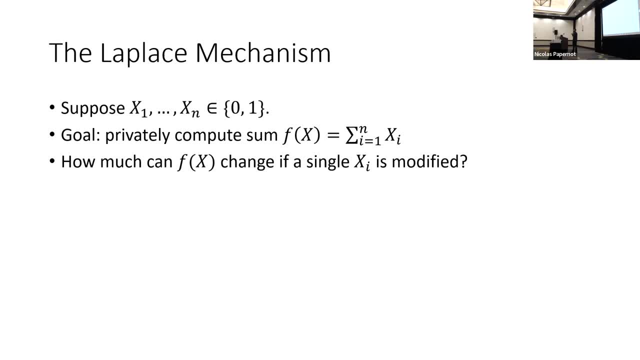 if a single data point is modified, And you can see, in this case, if you think about it, thinking about an arbitrary data set, you can really change a 0 to 1, or maybe change a 1 to a 0. But if you 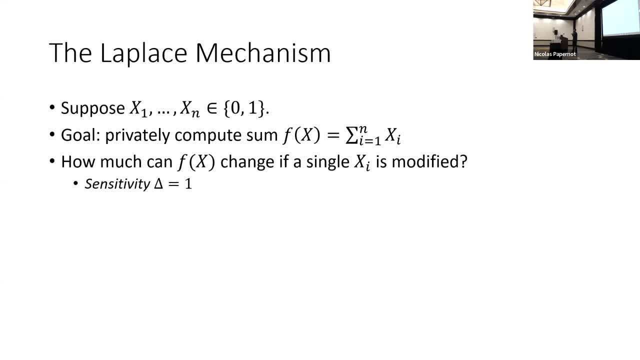 think about the sensitivity. it's just going to be 1. It's a very, very insensitive function And intuitively, this is an important quantity in differential privacy, because you know, we're trying to hide individual contributions in some rigorous way. So if a function is insensitive, 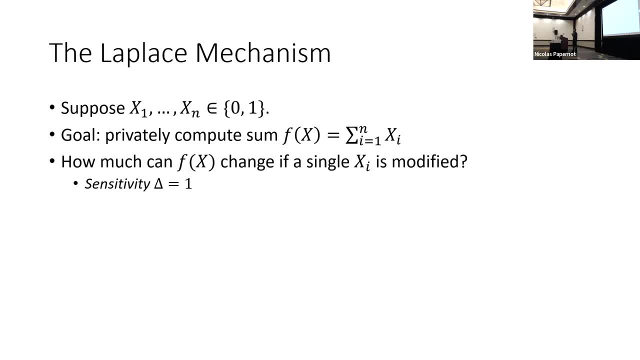 that means it's easier to privatize, intuitively speaking, Whereas if it's very sensitive it jumps around a lot. If you change one person's data point then it's going to be harder to privatize, But luckily in this case it's a fairly insensitive. You know it can change by just one. 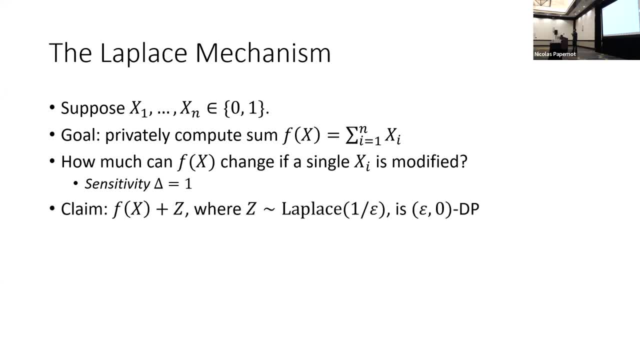 not too big in this case And my claim differentially private algorithm. what you do is you take your function, your sum function. here you add noise which is distributed to the sum function and you add noise which is distributed to the sum function. 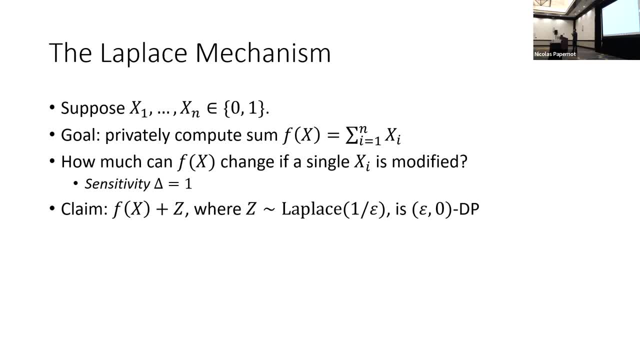 According to the Laplace distribution, which I'll tell you in a sec, And my claim is that this is epsilon 0, differentially private. So Laplace noise, that's the PDF, But maybe you know the way to think about it: is a two-sided exponential distribution. Exponential distribution. 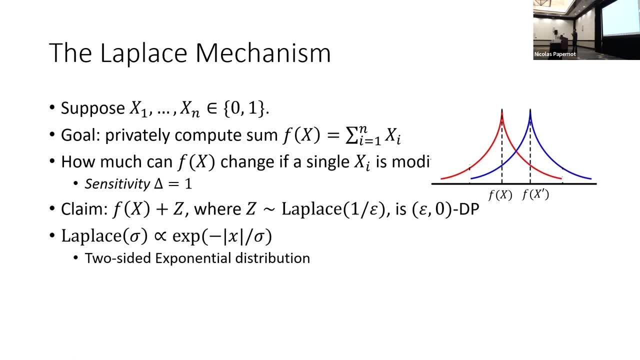 goes like this: You just mirror it on the left and right. So yeah, this is how you privatize a function. You add noise which looks kind of like that. you know curve right there. So you know these, right here are the two-sided exponential distribution And you can see that. 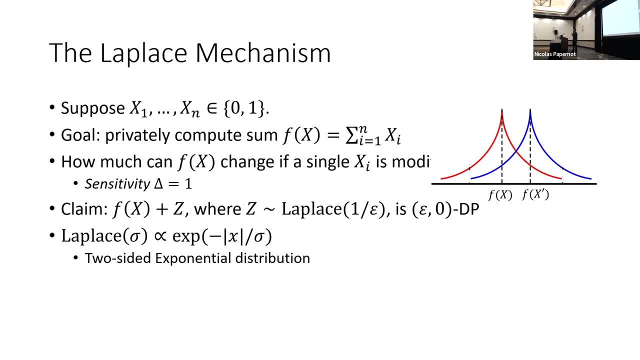 right here in fact are: if you had the value f of x, then you wouldn't just output f of x, you would output a sample from this orange distribution. Similarly, if you had f of x prime, you wouldn't just output f of x prime, you'd output a sample from this blue distribution. 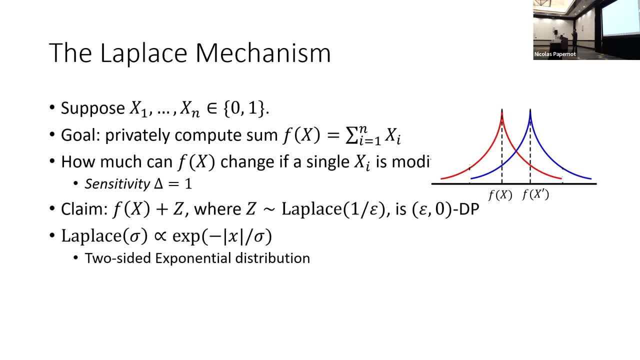 So I'll just comment on that as a sort of aside. Differentially private algorithms are always going to be basically samples from a distribution. You output a random draw And I'm not going to prove to you why this is differentially private. Here's a proof by picture, if you really stare at it. But 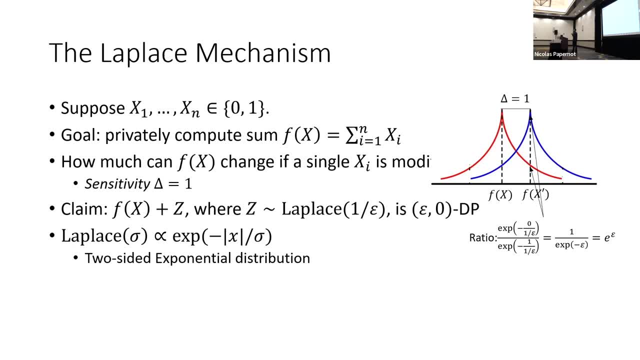 the point is, the PDF ratio here is bounded by e to the epsilon and therefore it guarantees exactly that definition that I showed you before. But yeah, if you stare at this picture long enough, maybe it'll make sense, But I'm not going to go too into that And let's make it a little bit more concrete. That's the idea. 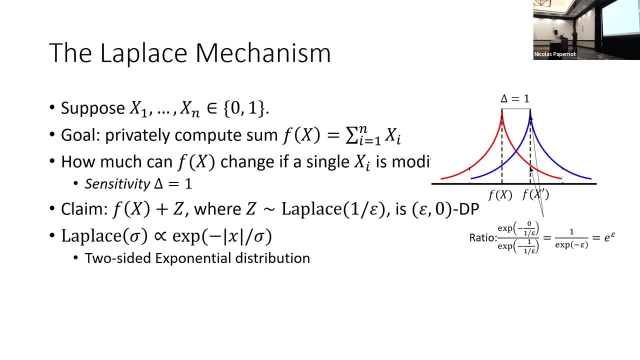 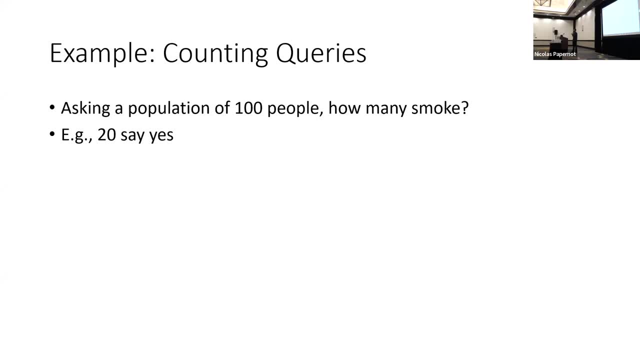 We take the sum and then we add Laplace noise. So to make it concrete, imagine, you know the same example- how many smoke? Suppose 20 people. that is f of x equals 20.. And you can guarantee 1 comma 0 differential privacy by adding: 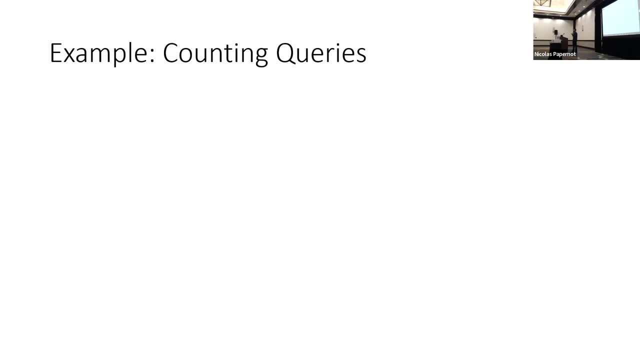 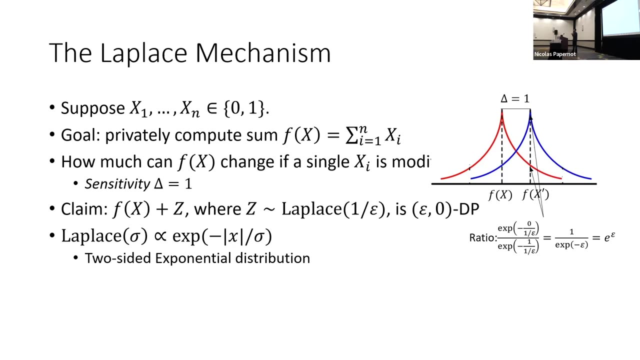 Laplace noise. So you can guarantee 1 comma 0 differential privacy by adding Laplace noise. Oh, one thing I want to really say here is: note that you know this is a quantitative definition in the sense that if you want stronger privacy, that is, epsilon being smaller, then you would add: 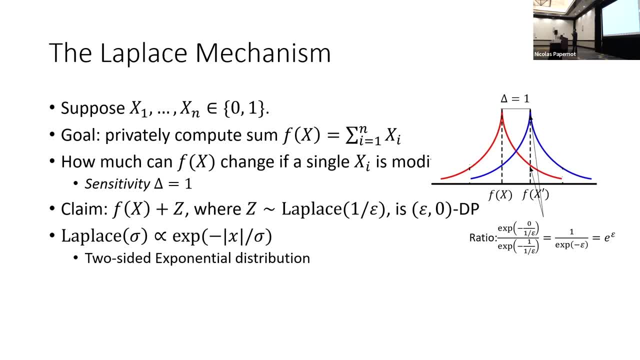 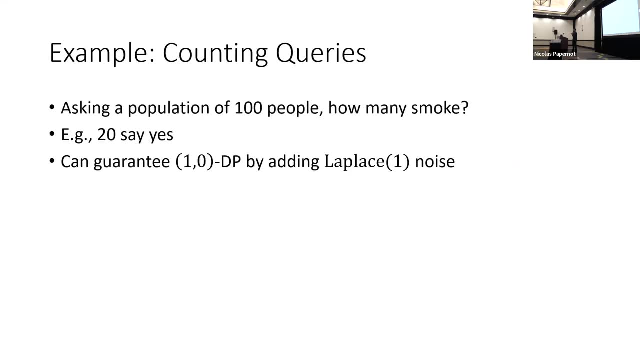 more noise. Say, you know, 1 over 0.1 would be Laplace 10, which is more noise, Whereas if you have a larger epsilon- say even epsilon equals infinity- then this would be a smaller standard deviation of the noise that you introduce. So, essentially, more private introduces more noise. 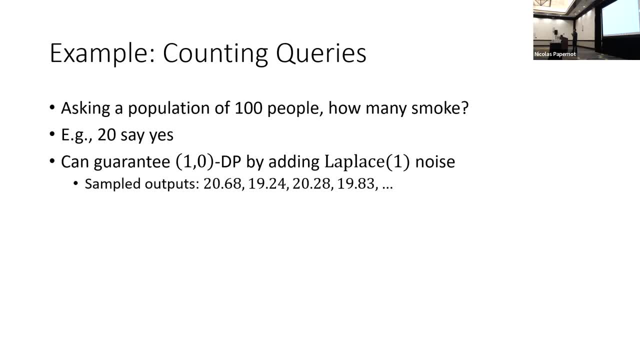 whereas larger private introduces less noise. So if you have a larger standard deviation of the noise, less private introduces less noise. So this is one example And I did a few samples, And for example, this 20,. when you privatize it using epsilon 1 comma 0, differential privacy, you get 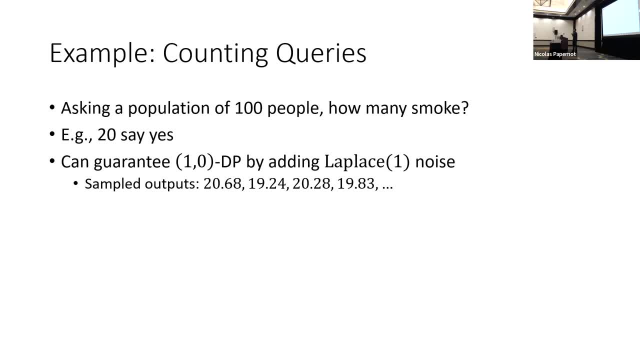 things which are pretty close to the right answer: 20.68, so on. But suppose you want stronger privacy, You want to get 0.1 comma 0 differential privacy. Then you have to add more noise of magnitude roughly 10.. And some samples from the output you can see here. some are pretty good. 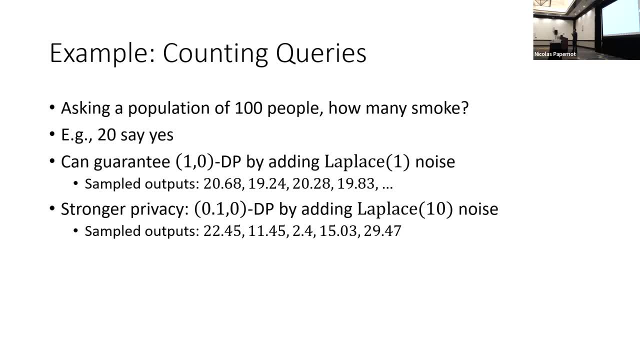 22.45 is pretty close to 20.. Some are much smaller, Like 2.4, which is natural. You wanted more privacy. you're going to get worse accuracy, And that's a common tension in differential privacy- Cool, So this is the Laplace mechanism for this. 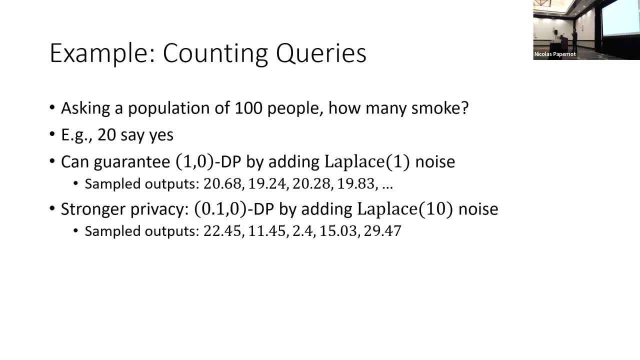 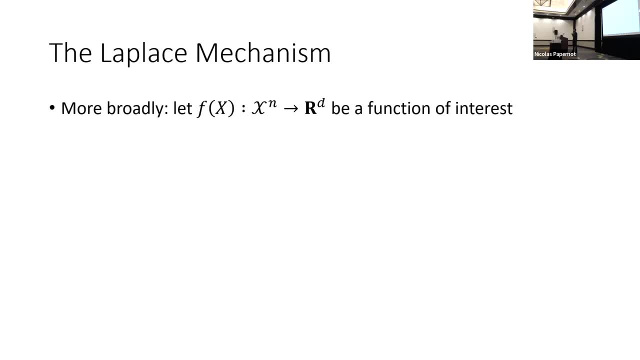 simple example. Let's make it a little bit more general than just adding sums. I'll try to state it in its full generality. Suppose you have some function of interest which takes in a sensitive data set and outputs, say, a real vector. So now we're not just going to be focusing on a sum. 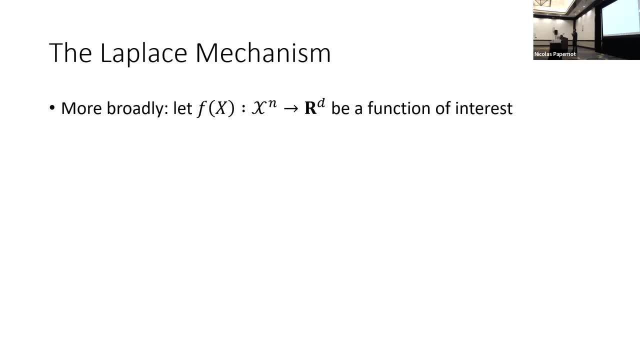 or sorry, on a one-dimensional sum. It could be anything that maps, which would be a dimensional vector, And we're going to let this quantity here be the L1 sensitivity. That's a mouthful, So think about it in terms of these words. The math backs it up. 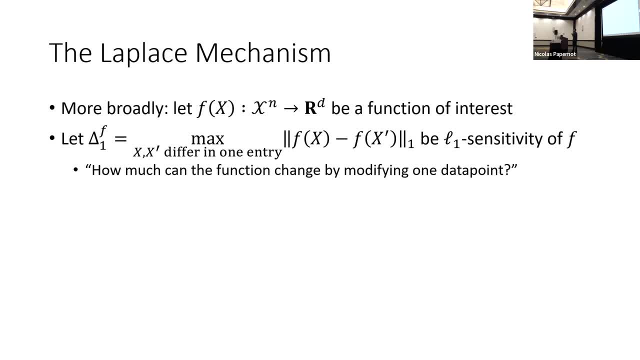 But how much can this function that we care about change if we modify one data point And so notice that this is a worst case over every single data set and every data set that could be neighboring to it? So really, looking in the worst case, how sensitive could this function be, Like we saw? 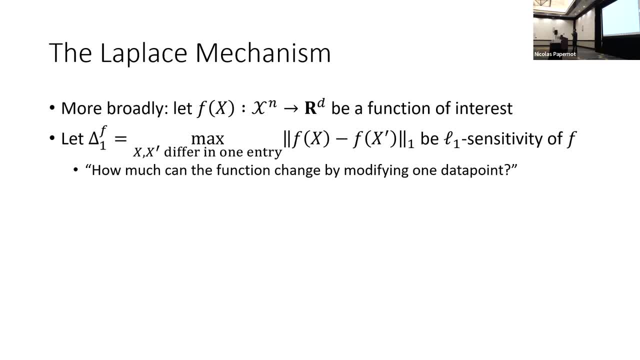 with zeros and ones, but in general it could be much larger. And in particular we measure how big the function difference is in the L1 norm And here's the sort of general Laplace mechanism theorem, which is that if you take your function and you add Laplace noise to each of the coordinates, 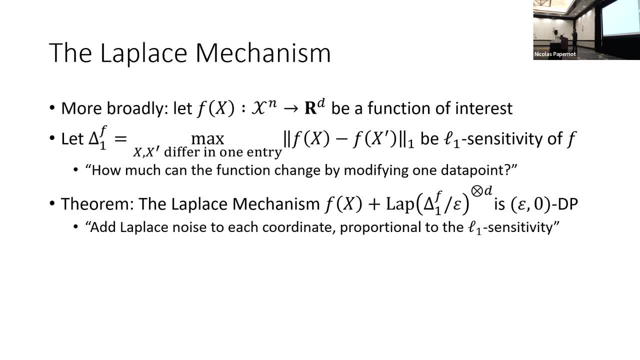 in words I say here: yeah, you add Laplace noise to each of the coordinates, then this is going to be epsilon zero, differentially private. Just to emphasize how big the noise is, you'll note that in the numerator of the size of the noise is the L1 sensitivity. So that kind of. 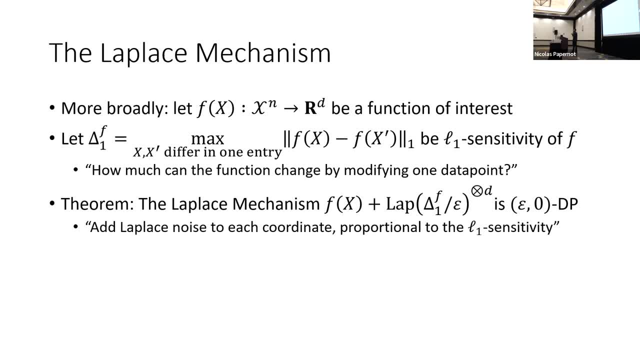 matches the intuition I said before, where if it is more sensitive, then you have to add more noise, because it's harder to privatize, Whereas if it's less sensitive, then you have to add less noise. Similarly, once again, when you want epsilon to be smaller, that necessitates more noise. And 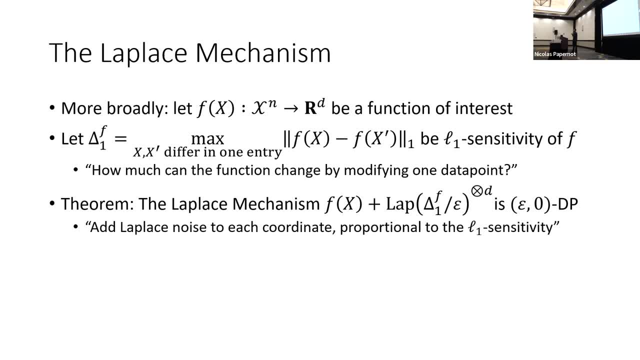 if epsilon is larger, that necessitates less noise. So the magnitude of the noise kind of matches on those two things that we care about. It's bigger if you have a sensitive function or if you want stronger privacy guarantees- Cool, And just to make this one a little bit more, 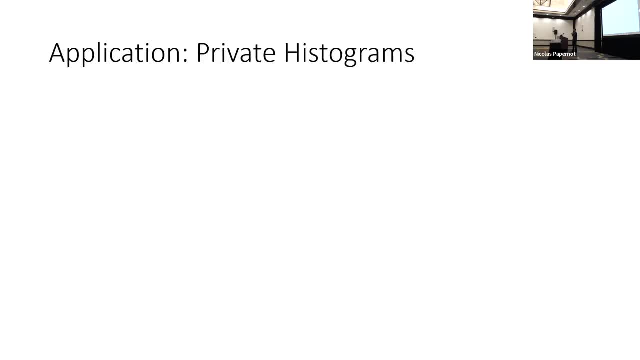 concrete. I'm going to give you an example on private histograms. There's a very common thing that you'd want to know for a data set: you know number of data points that fall into each of K categories. Say like: here is a data set and someone's weight in pounds, and you know. 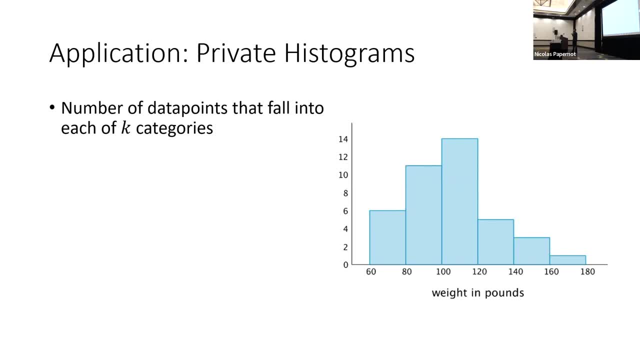 this is what a potential non-privatized data set could look like, But of course, maybe weights are sensitive. so maybe you want to privatize this histogram, And I'm not going to go through the details, but essentially the Laplace mechanism you can privatize this by. 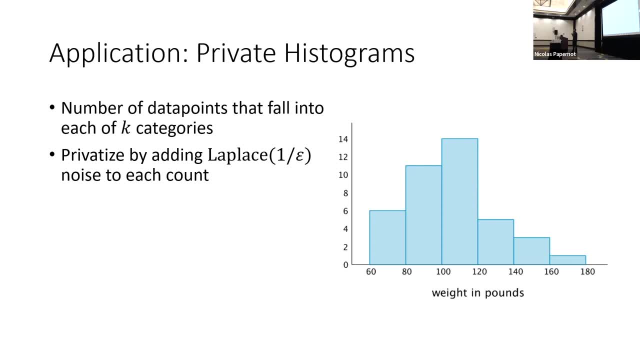 adding Laplace 1 over epsilon noise to each of these different counts, Each of the bins is essentially perturbed And you know you get something that looks like this, for example: You can see how it changes from the original counts to something a little bit different. Some: 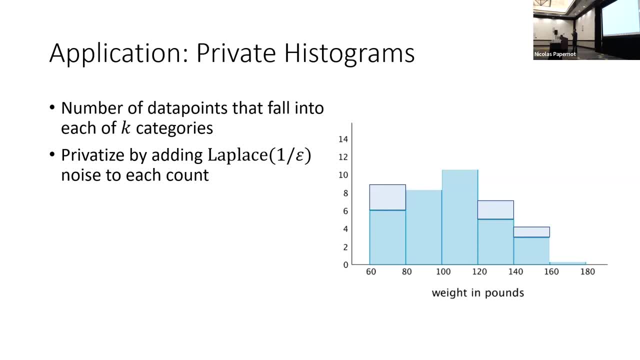 numbers went up, some numbers went down, But if we work through the analysis, you'd see that this is differentially private And then you can release these. you know privatized counts for someone to do data analysis on. Yeah, I claim that they are going to be epsilon zero dp. 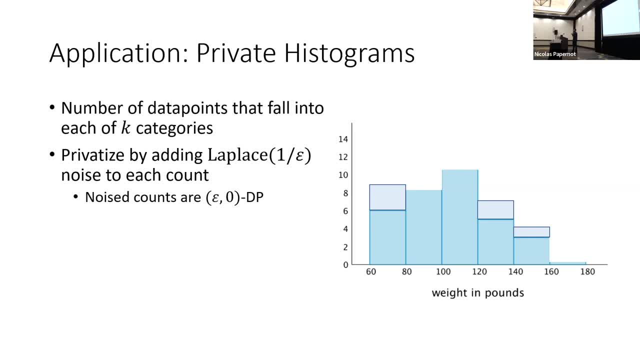 Cool. So Laplace mechanism is the first thing everyone learns and it's kind of the most useful one. Sorry, I won't make such a strong statement. There's lots of useful algorithms And another useful one, which is very similar, is the Gaussian mechanism. You know this is very similar to before. 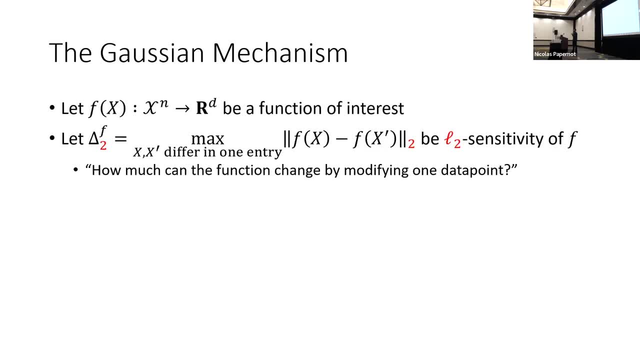 so I'm not going to, you know, go into all the details, But it's almost identical. I highlighted the changes in red. Okay, But the thing I want to get away here, the thing I want you to take away here, is, instead of adding Laplace noise, 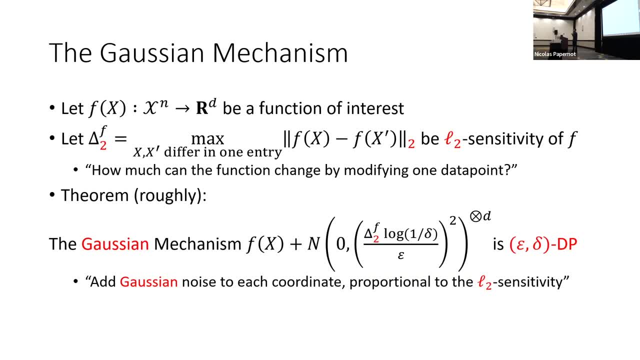 which is, you know, very sort of. if you're not familiar with differential privacy, you might be wondering why Laplace noise? And the reason is because it fits the definition perfectly and kind of works for that. But another common thing you might do is adding Gaussian noise, And essentially this slide says that you can add Gaussian noise. 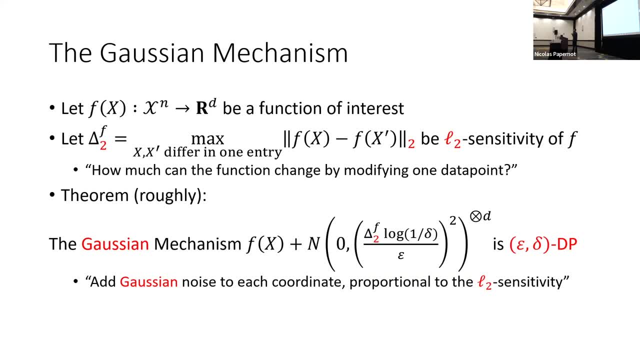 instead of Laplace noise, and it'll still be private, And I could walk you through. you know all the terms, but the same sort of things happen. So I'm going to take a moment to highlight the differences here and then talk about. you know what the difference is between the Laplace and Gaussian mechanisms. 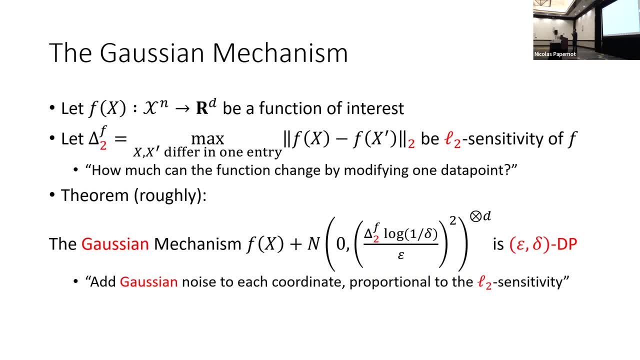 In particular, if it's more sensitive, then you have to add more noise to guarantee privacy, and so on. There's two differences I really want to highlight here. I have some Gaussians. You know what a Gaussian looks like. probably The main thing I want to highlight here are the difference between the Laplace and Gaussian mechanisms. 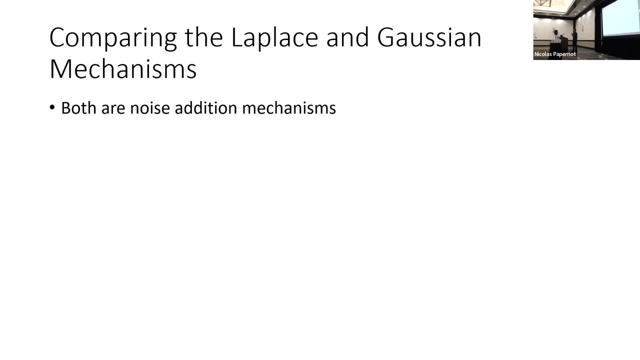 So the similarity, first of all, is like, like I sort of said, they're both noise addition mechanisms, That is, you take the function, which is non-private, and you add Gaussian noise, and you add noise to it either from a Laplace or Gaussian distribution. 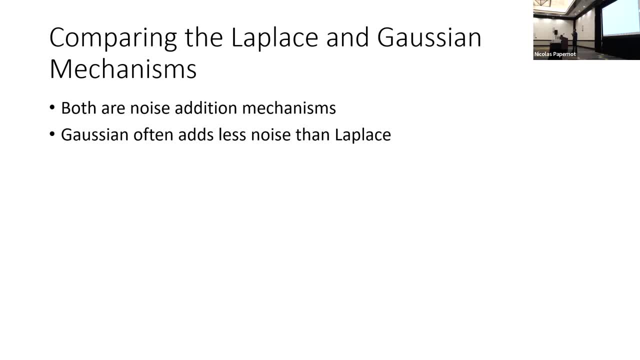 So it's similar in that way, But the difference is that the Gaussian distribution, the Gaussian mechanism, it often adds less noise than Laplace, And the reason is because one of the details which I didn't say in the last slide is that, interestingly, you add noise according to the L2 sensitivity rather than the L1 sensitivity. 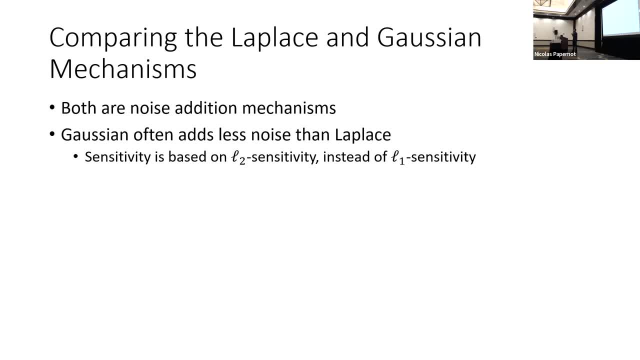 And just one fact which may not be obvious to everyone is that the L2 norm is always, at most, the L1 norm, So therefore there's going to be less noise added. On the other hand, while it essentially necessitates less noise, 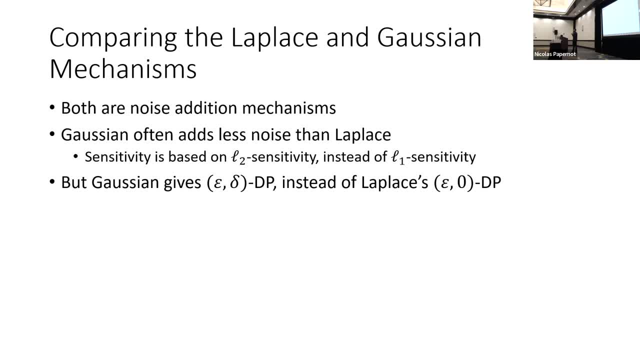 the downside is that it gives you a weaker privacy notion. that is known as epsilon delta dp Instead of Laplace. the Laplace mechanism is epsilon comma zero dp, So it weakens your privacy notion, but you add less noise. I didn't really tell you, like you know. is that a bad thing? Is that a good thing? 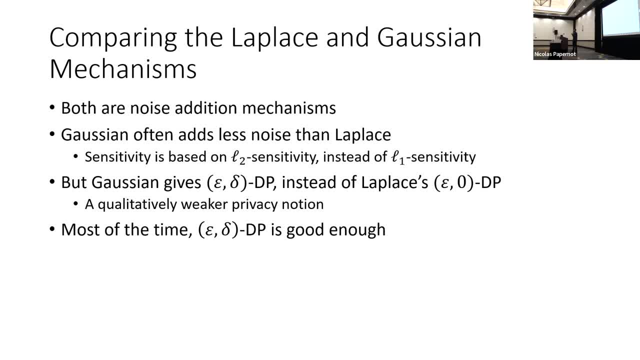 I'm going to claim that most of the time, epsilon delta dp in most applications is going to be good enough, In particular, if you're asking a lot of queries on the same data set. you know, maybe you want to do more than just finding out how many people smoke in a data set. 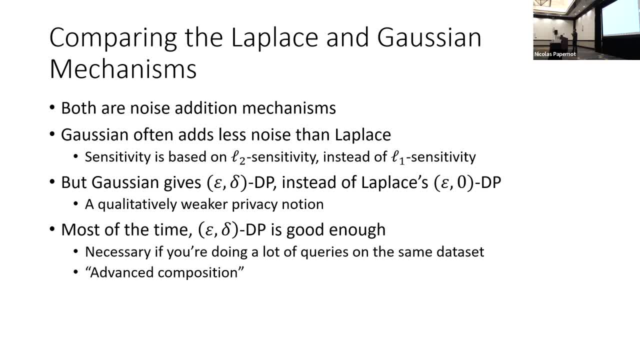 You want to do many queries, Then you're going to use something called advanced composition, which necessitates a prox, dp, which we'll talk about in a few slides. But really the point I'm trying to get at here is that, yeah, 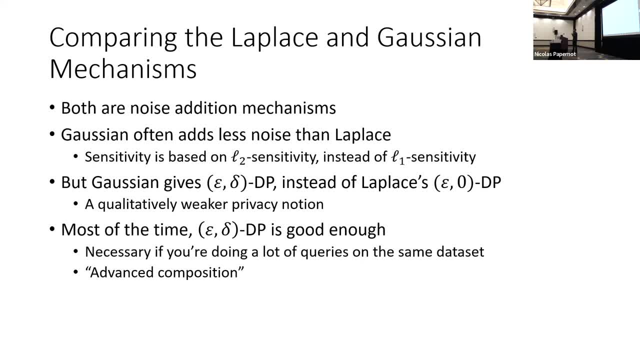 the Gaussian mechanism for many intents and purposes is good enough. In particular, we'll see when we're using it, when we're training a machine learning model privately. that's kind of the only way that we're going to do it. 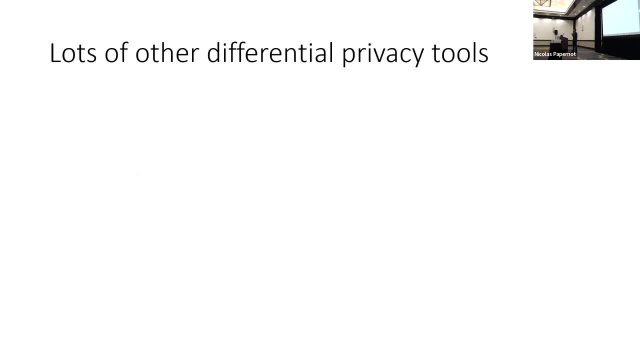 Cool. So these are just two basic mechanisms and you might be thinking that, okay, you've taught me two things which are you know, you take a function, you add noise is everything in differential privacy just doing noise addition. 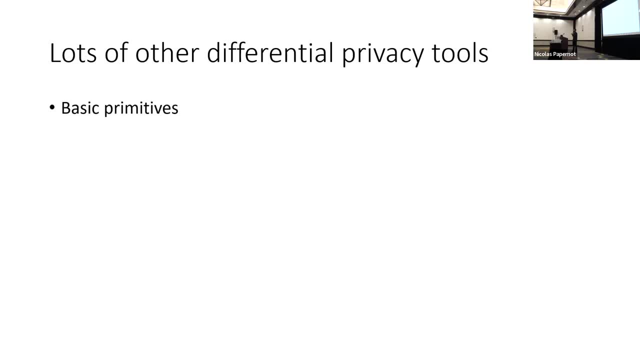 And the answer is no. There's many other things which I don't have time to get into. There's one thing you know. it was heartbreaking. I had to cut the exponential mechanism, which is my favorite. LLT It's called algorithm in differential privacy. randomized response is another kind of different thing. sparse vector. 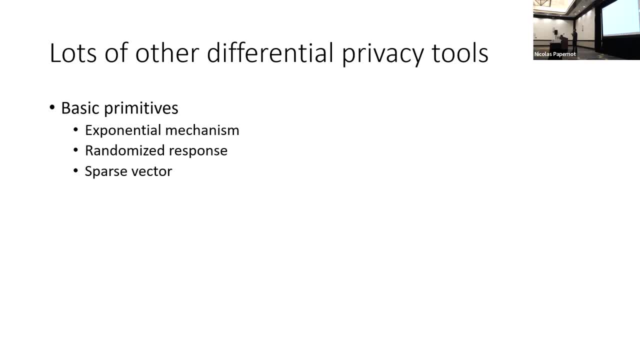 These are other primitives which are commonly used and you know basic tools in your arsenal that you should have if you're doing differentially private algorithm design, And these are nice to have in your toolbox because they're useful in building more complex procedures. 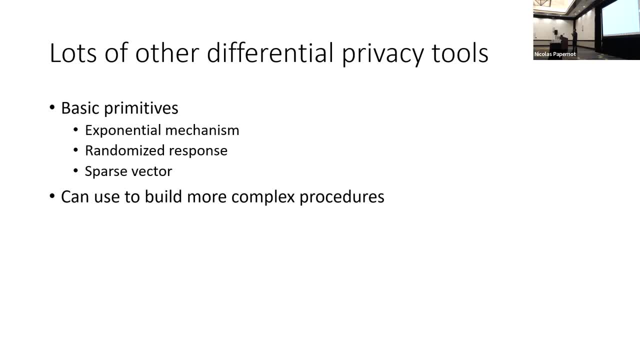 And, as I'll sort of explain, you can put these tools together in the right ways and they'll give you something more mature and sorry, allow you to build basically a more complex system which does more than just output. you know how many people smoke privately? 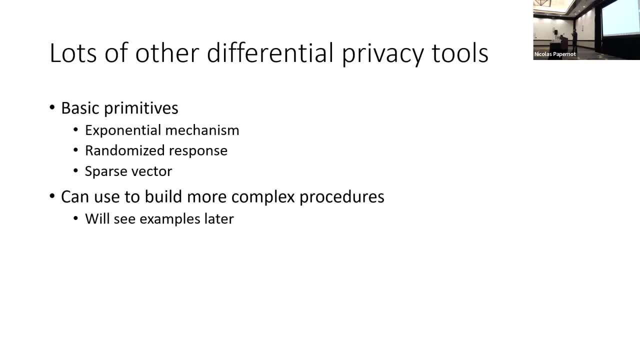 And we'll see some example of that. But hopefully I've gotten across to you in this segment that there's some very simple algorithms which guarantee differential privacy in simple settings. That's great And, like I said, I promised you we'll be able to do something useful with these, which is more complex than just sums, but we'll put a pin in that. 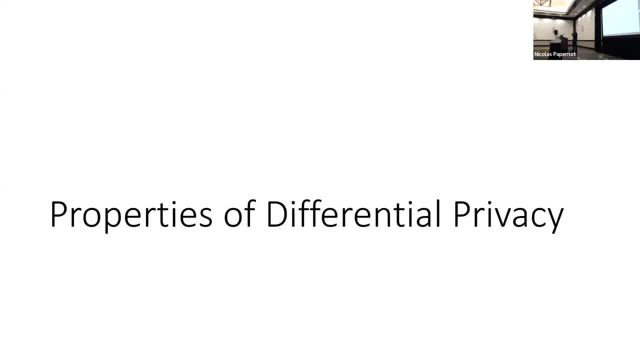 Cool. So for the next segment, I'm going to talk about properties of differential privacy, That is, you know, we have this definition, we have some algorithms, but if that was it, then it would be restricted to doing very basic things. 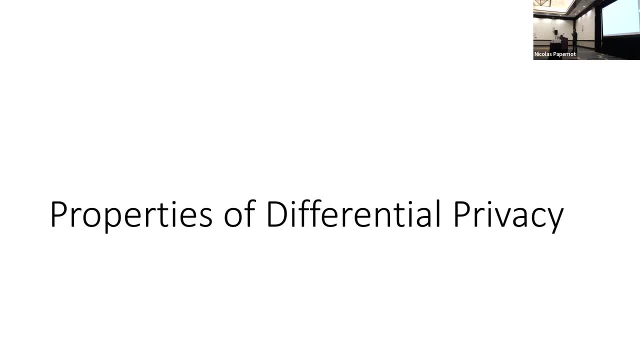 So I'm going to tell you some convenient properties which make it very user friendly in my opinion, And there's three properties I want to focus on. One is called post processing, And in words this says you can't undo privatization of something which is released under the constraint of differential privacy. 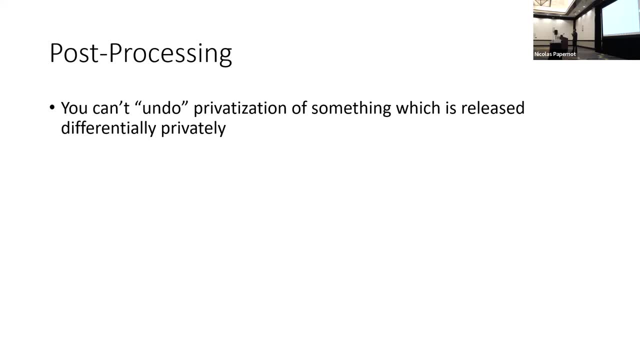 So, just like that, differential privacy. So what that says is: you know, suppose we started with 20 people smoked in the data set and we add noise and it says 22.47 people smoked. There's no way given if I. 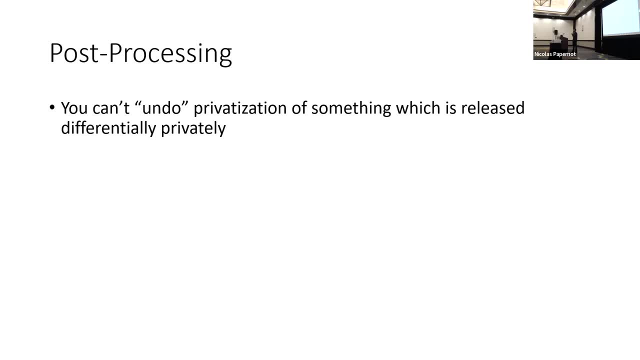 give you the 22.47,. there's no way you can like stare at that really hard and say, oh, there must have been 20 people actually in the data set. You can't undo privatization. Yeah, basically you. 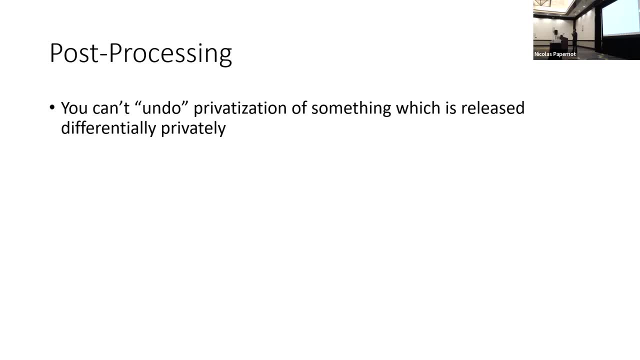 know. every once something is released privately into the wild under differential privacy, that guarantee just holds. And the more mathematical way of saying this is as follows: If we let m be a differentially private algorithm and f is just something which is arbitrary, it's an arbitrary. 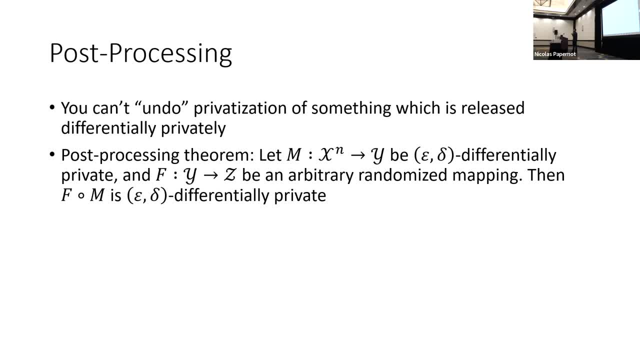 function, then if you compute m on some data set and then compute f on the output, that's going to be differentially private as well. So it's saying you know the composition of any function. so I'm not gonna use the term composition because that's confusing for what I'll say later. but basically, 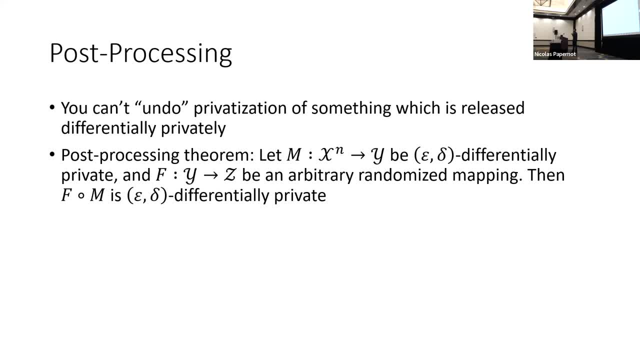 running an arbitrary function which doesn't look at the data again on the output of a differentially private algorithm is not going to somehow magically violate privacy. So that's very convenient because we'll see later. you know we're going to train a machine learning model. 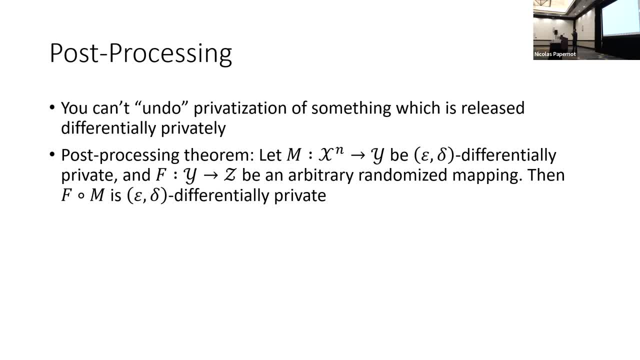 privately and then after that we're going to give it to the users. they can do whatever they want with it, and we still have the very strong guarantee that we're not going to reveal things about the training data set. So this is a very important property. Another thing is group privacy. 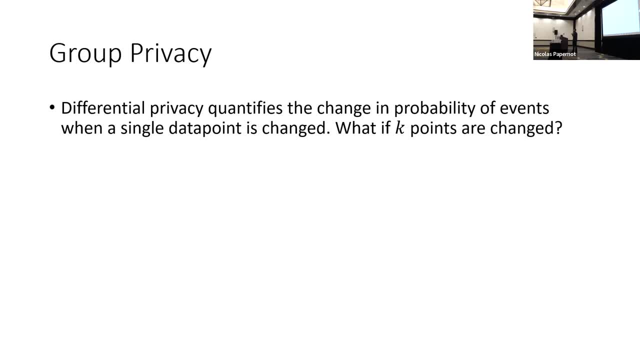 Now, if you have, say, neighboring data sets, you know one data point is added or removed, one data point is changed. but what if K points are changed, For example? you know, maybe two people are uncertain about whether their privacy will be preserved together. maybe jointly their privacy could be. 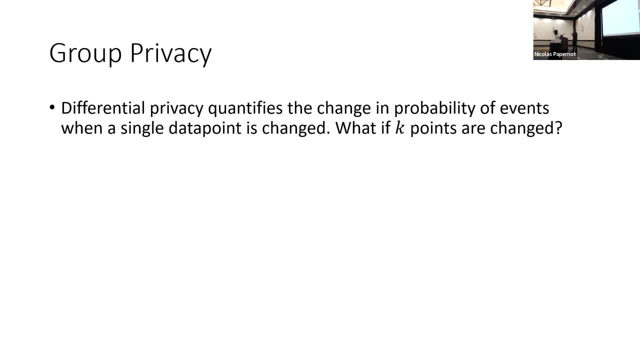 violated. But the nice thing about differential privacy is just by reasoning about neighboring data sets, the privacy loss degrades gracefully when you consider things which are maybe two spaces away or three spaces away or something along those lines. so that's kind of a good thing to think about. 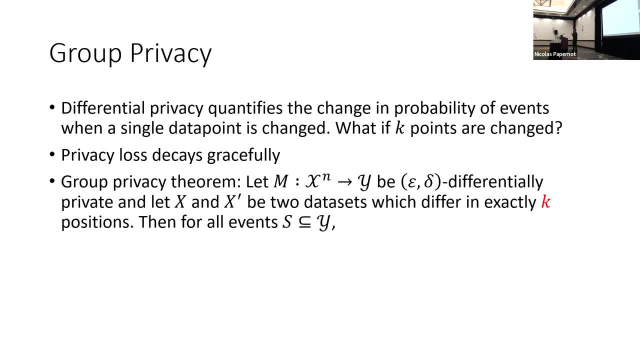 space of the way, There's maybe multiple changes. And here is the group privacy theorem, which is it's going to look very similar to the definition of differential privacy. So it's a little bit of a mouthful in the exact same way. Don't focus on too much of it. In particular, ignore this term. 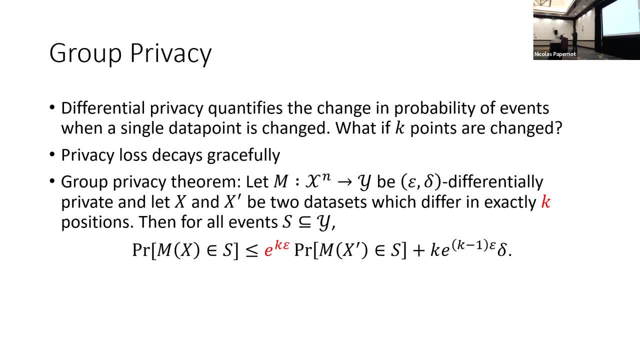 over here. The main thing I want you to focus on is the fact that instead of differing in one entry, we're saying that x and x prime differ in k entries, And then instead of having e to the epsilon here, we have e to the k epsilon. So this is kind of the natural thing that maybe you would. 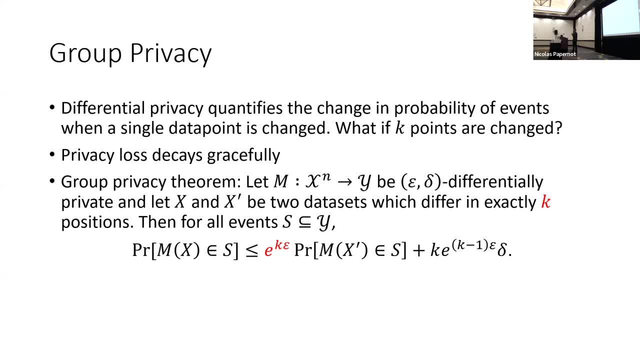 expect. You know, if you said k equals to one, then this just recovers the original definition of differential privacy. But you know, allowing more changes weakens the privacy guarantee in some sort of predictable and smooth-ish way. Cool Of these three properties. 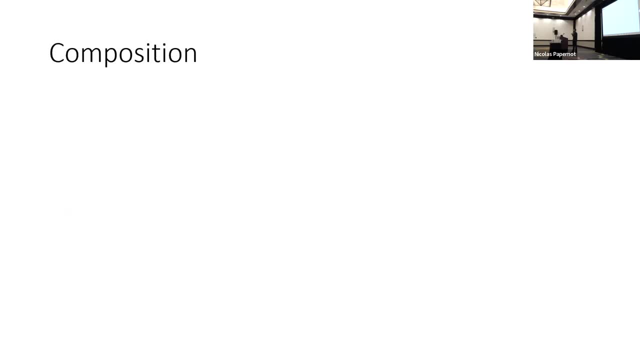 I'm going to show you. this is probably the least important, but it's still an important one. The most important one by far in my mind is composition. Composition is a very, very powerful property which lets us do things with differential privacy. If it didn't exist, 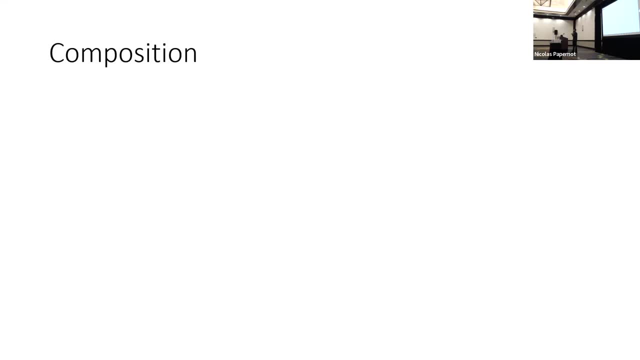 then we'd be stuck with very basic things like you compute one sum and then you give up. You're done Like the intuitive idea is suppose I ask you know multiple queries about the same data set. Say, I want to know how many women in my data set smoke, And then maybe I also want to know: 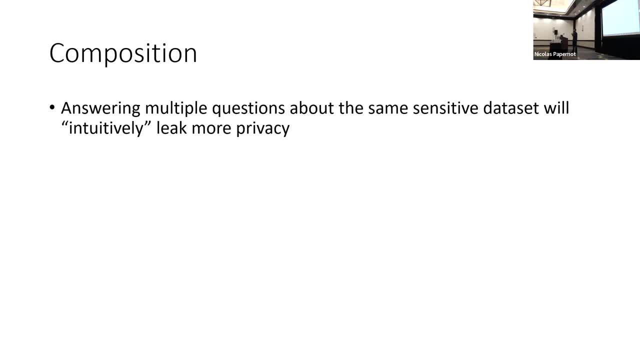 how many men in the data set are over 18.. Uh, up to 25 or something. If I ask multiple queries of the same data set, intuitively, somehow we're giving out more data about the sensitive data set And therefore you know the privacy. 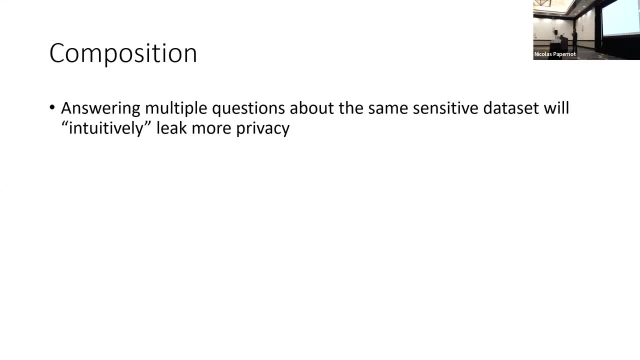 weakens when we do multiple queries. but it's unclear, It's not immediately obvious how to quantify this sort of thing. Like if I do, uh, three disclosures which are differentially private, then what happens? Is that still differentially private or not? 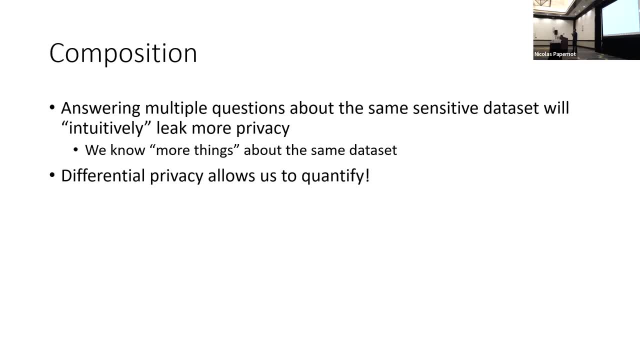 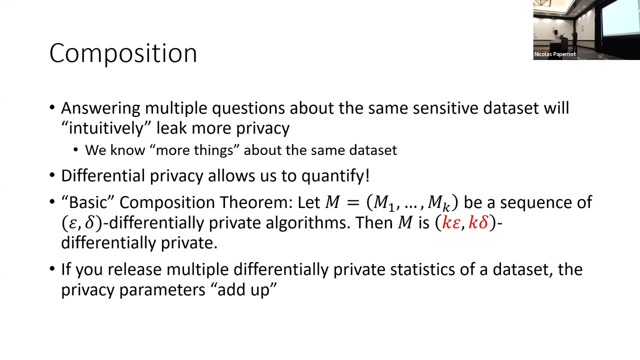 And, uh, the nice thing thing is that differential privacy- this is why i think it's so useful and powerful- is because it allows us to quantify how things uh degrade when we have multiple queries on the same data set. so here is the basic composition theorem uh, which you know. the plain text description is below: 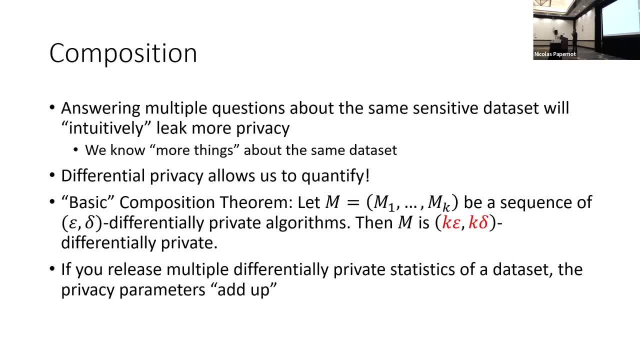 basically suppose you have a bunch of differentially private algorithms and you run them all on the same data set and you release all of their outputs, then the result is going to be basically what you would get by adding up the privacy parameters. for example, suppose they're all epsilon, delta differentially private, then uh k algorithms run will be the overall. 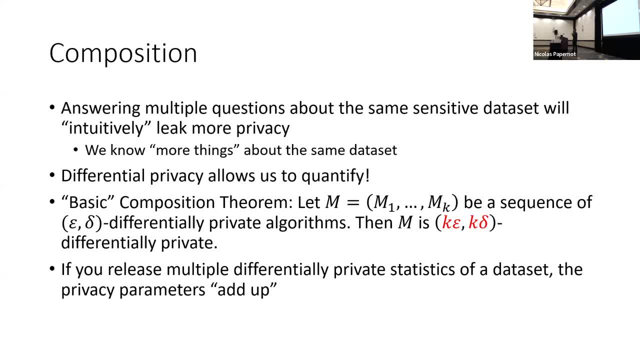 release of all of those will be k epsilon, comma, k delta, differentially private. so this is, you know, very convenient, because, like that, if i had to, if you had to guess how the privacy would be leaked- uh, how the privacy would degrade by multiple outputs, it's exactly what you probably would. 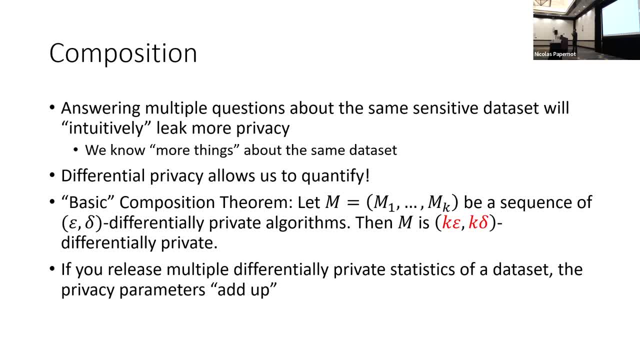 guess, you know, you just add things up and it works out very nicely, you? so let me give you an example. uh, you know, i'll mention again like: this is what's going to be really the workhorse, something like this that allows us to build more complex procedures, rather. 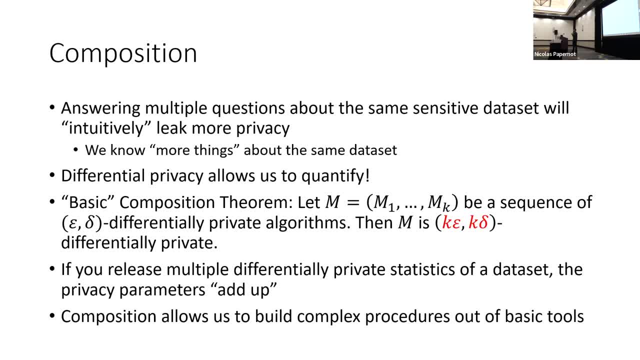 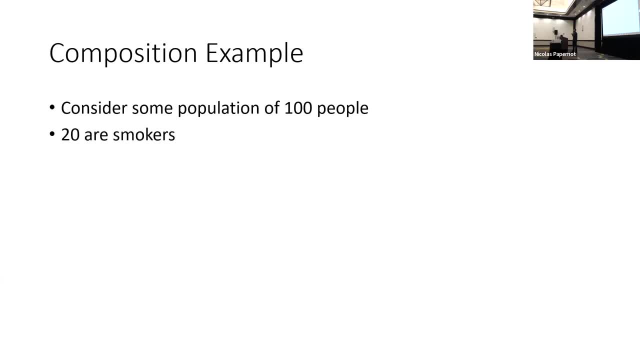 than just uh, releasing, say you know, sums. but one example i want to give you is: for example, is there the population of 100 people and say you know, first of all, we know 20 of them are smokers. we can privatize this uh with laplace: one noise and we get, say, 19.51, suppose, additionally, 37 have some sort of chronic illness. privatize this, we get 36.89. and 12 people have a high income of at least 250 000 a year and we privatize that and it gives us uh, 12.53. let's say now my claim. 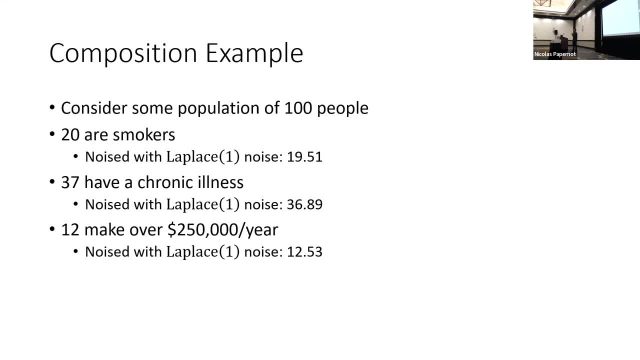 is that if we release, if we release each any one of these in isolation, that would be one comma zero, differentially private. but since we're releasing these three statistics, which are each one comma zero differentially private, the overall release of these statistics is going to be one comma zero. 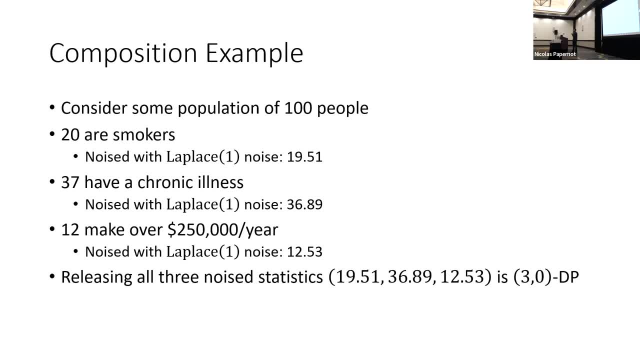 differentially private. but since we're releasing these three statistics is going to uh give three comma, zero differential privacy. so yeah, it shows how you can add. you can ask multiple queries on the same data set and quantify how much you know how private that is or not. the downside is that 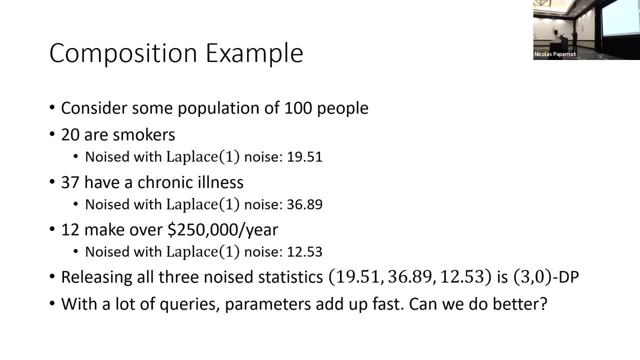 these, these add up really fast. uh, in the sense that if you do a hundred or a thousand or a million queries, then you pay a million times the privacy cost in these parameters and that can add up really fast. um, there are some cases where you can do a hundred or a thousand or a million. 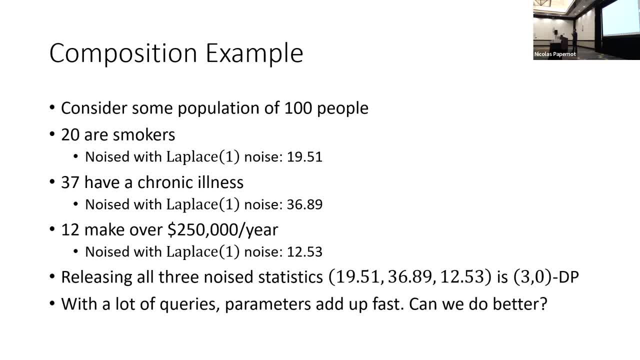 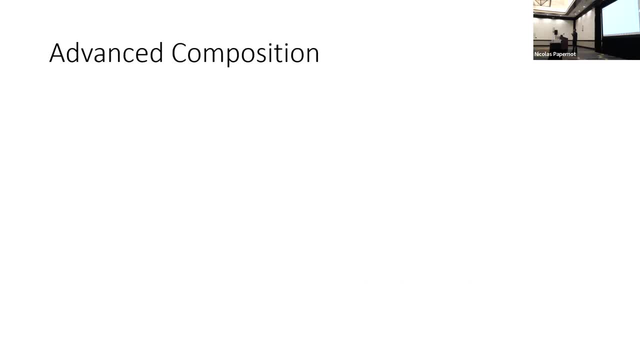 this is where, uh, we'll get into. you might want to do many, many queries on the same data set and therefore, this is uh, this is not good. can we do better? and fortunately, yes, the answer is yes. there's some tool called advanced composition, which essentially allows us to ask more queries. 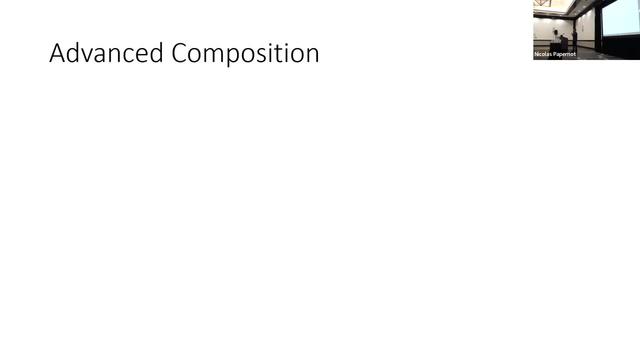 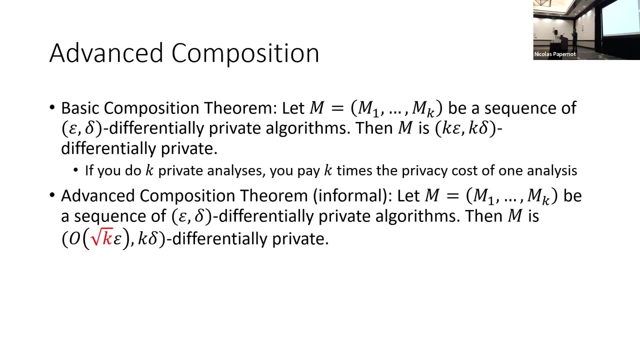 for the same uh for the same uh privacy cost. so i'll just, you know, flash this, the basic composition which i had before, where the parameters add up. here is the advanced composition theorem, which, uh, is a little bit informal. there's some detail i'm hiding- but, very roughly speaking, by 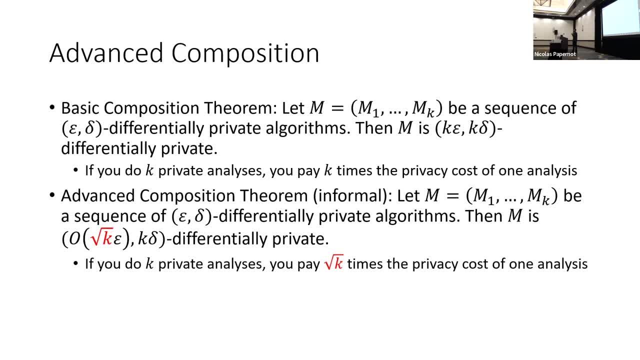 more careful analysis, you can actually show that instead of just adding up the parameters, you know paying a cost of k, then you can pay a cost of square root k instead, which is in many cases dramatically smaller, for example, just to give a kind of quantitative comparison. this isn't totally. 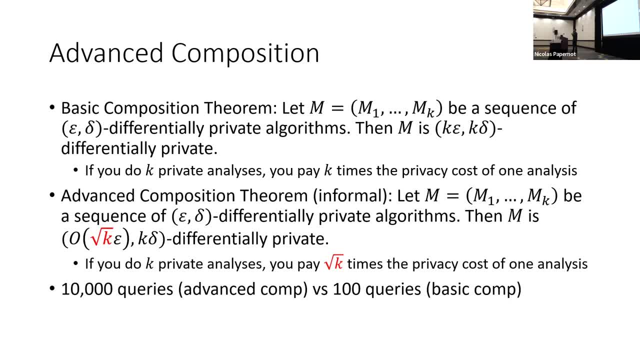 precise. suppose, uh, if you do a hundred queries on a data set, if you just use basic composition, then for the same privacy cost you can, uh, do 10 000 queries using advanced composition, roughly speaking, not not totally accurate, but something along those lines. so this shows you. 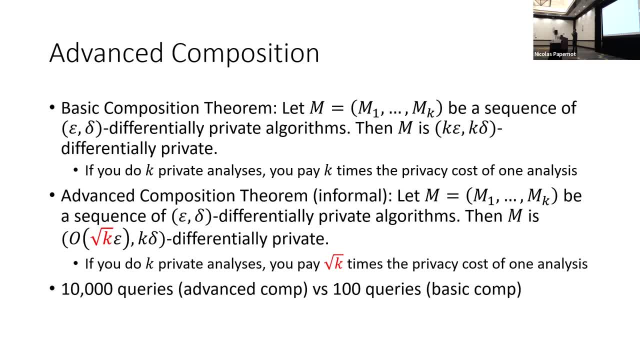 that, essentially, you should, in most cases, be trying to use advanced composition when you have many queries, because this allows you to do more analyses on your data for the same privacy cost that you would get under basic composition. and this is really, really, uh, powerful and important, the fact that we can do. 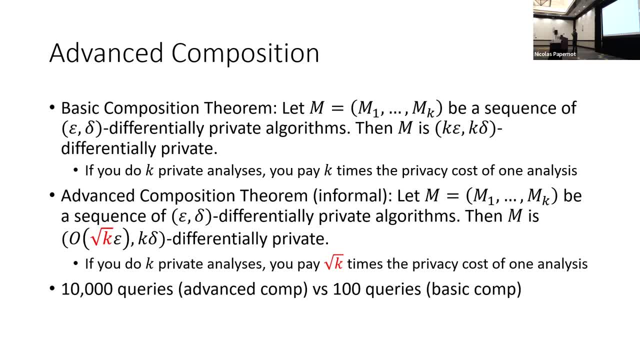 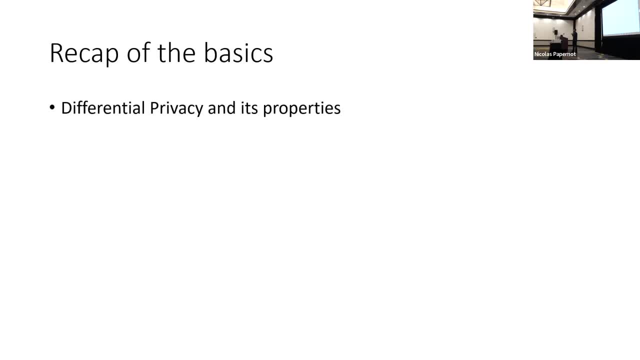 so many analyses on one data set, uh, without the privacy going totally out of hand. so, okay, let's recap, uh, what we've talked about so far. we've talked about differential privacy and its properties, like these things, as well, as you know, private mechanisms, including Laplace, and 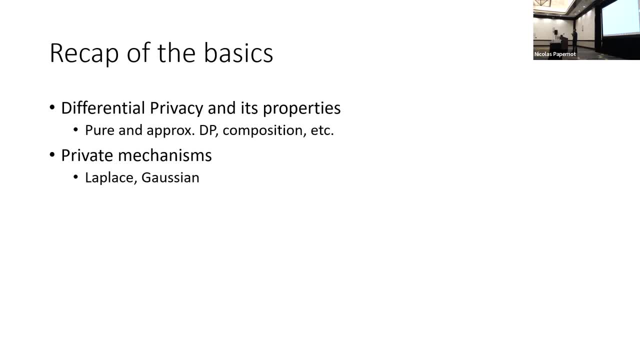 Gaussian mechanism. uh, now I want to fulfill the promise I made to you and show you some of the things you can actually do. so I'll show you briefly a few applications where differentially private, differential privacy has been used, and then, during the last segment, we'll show how to pray, uh, train a model under differential privacy. 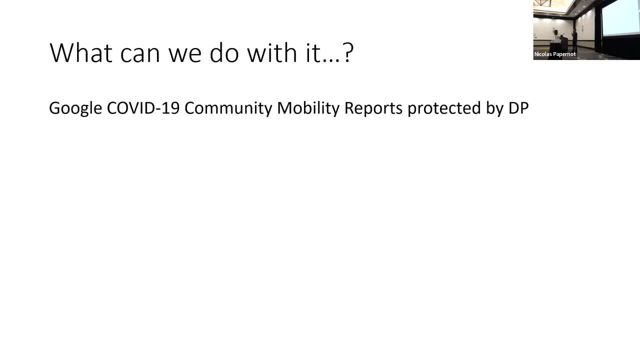 so some examples of where it's been used. this is one thing which uh, in the wake of coven 19, when it started, uh, Google started releasing these Community Mobility reports, which are uh differentially privatized. so what this shows is essentially uh, in various different locations, how many people were in retail and Recreation? how many people were? 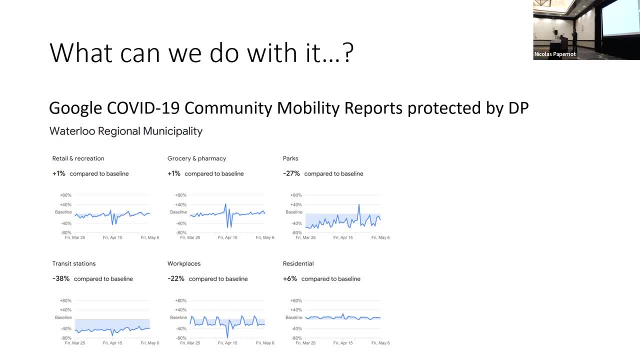 at transit stations. compared to pre-covered. you can see, for example, uh, not as many people were in transit stations in Waterloo region, uh, or workplaces, whereas more people were staying at home- kind of what you expect, um, but this uses people's location data, which is clearly very 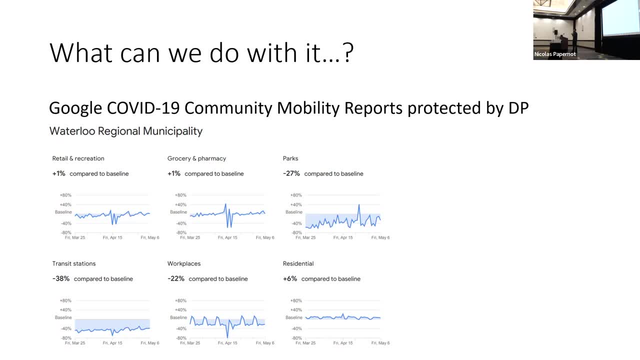 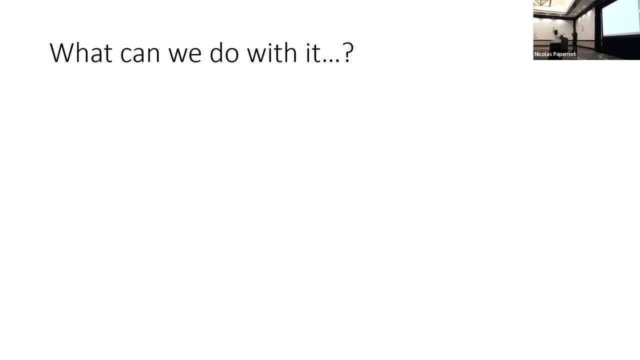 sensitive. you wouldn't want your you know location where you went all time of the day to be released, so they released these using differential privacy and that protects people's location data. when still finding aggregate statistics over a population of where people are going- another, uh, very high profile. 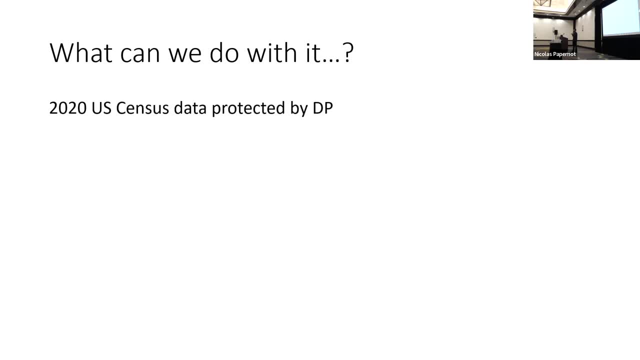 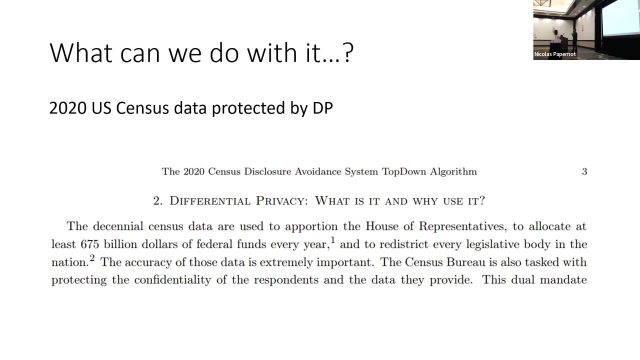 and perhaps I, in my opinion, the most important application of differential privacy so far has been in the 2020 US census. uh, if you were in the United States on April 1st 2020, your data was run through a differentially private algorithm. uh, and this is very important because, for example, it's 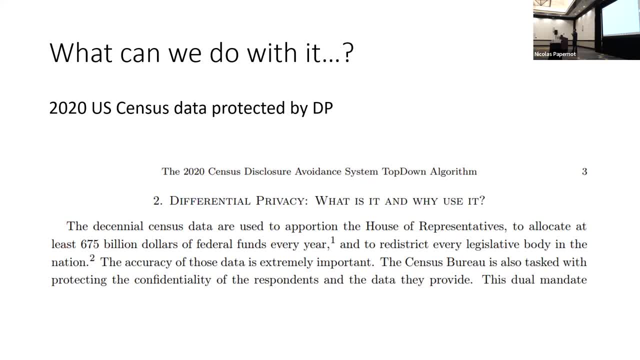 used to uh do- allocation of a lot of federal budget up to 675 billion dollars at least, at least that much, and uh you know. so there's a lot of uh. there's a lot of people who are depending very much on the uh outcome of the uh census information and, yeah, this has been a there's 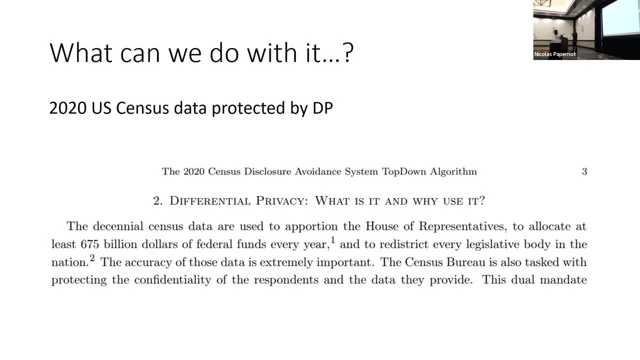 been a lot of- uh, you know- competing interests here. in particular, I think, uh, you know this is one of the few things in- uh, I'll not say that, but uh, there's literally been federal lawsuits involving differential privacy as an algorithm, uh, which you know some stakeholders feel like. 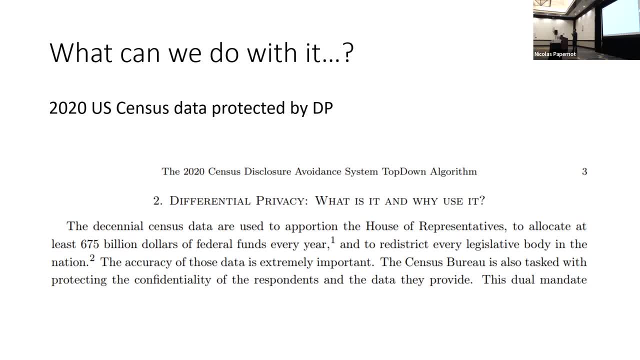 this is violating their ability to get uh their numbers, but if you want to preserve privacy, which the Census Bureau is mandated by law to do, this is kind of the way you have to do it. so this is an ongoing discussion, in fact, between social scientists and uh uh private and 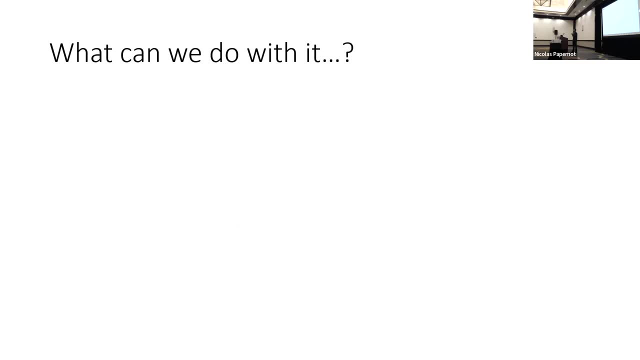 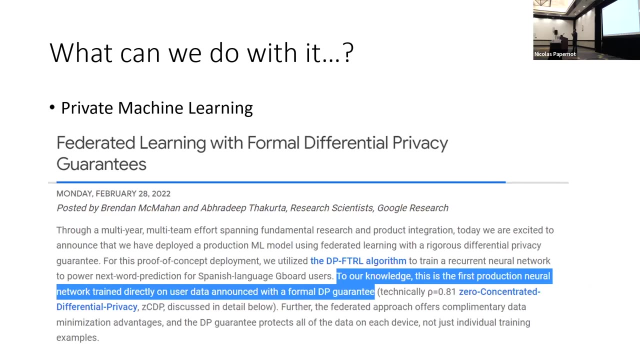 statisticians who are, you know, interested in furthering privacy. and the last one I'll mention is, uh, private machine learning, which will go into a bit more depth, but I thought this was really cool. uh, a recent deployment about a year ago. uh, where essentially the next word: prediction. 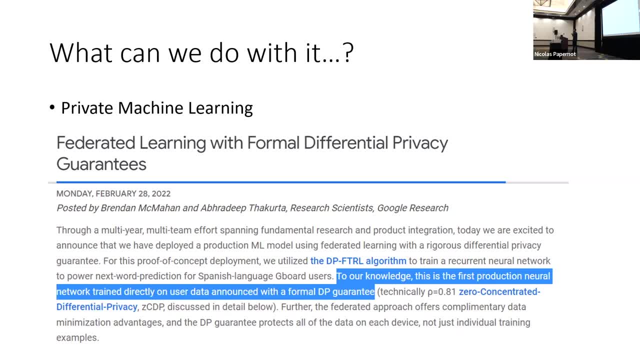 in the Spanish language: uh, Google keyboard, the gboard. uh, it is trained using differentially private, uh federated learning. well, we'll not worry about federated learning today, but, um, really using differential privacy guarantees and as to best of their knowledge in mind is the first production neural net trained directly on user data, announced with 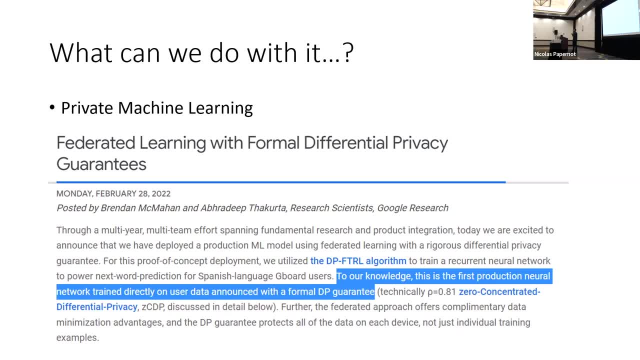 a formal DP guarantee. so, yeah, I think that's pretty cool that essentially, you know, even based on these simple things like you know- noise, addition and composition- they essentially built something on top of it which is able to work in your phone and give you private next word predictions. 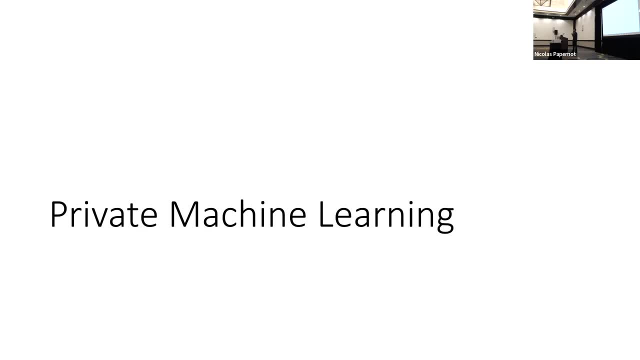 for the rest of this talk. I'll tell you, you know, some of ideas of how, uh, that's done. I'm not going to go into full detail and I'm not going to tell you specifically their algorithm. I'm going to tell you something a bit simpler, but it'll give you an idea how even these complicated machine learning. 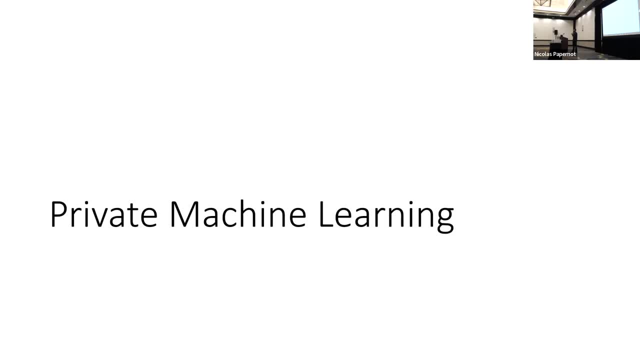 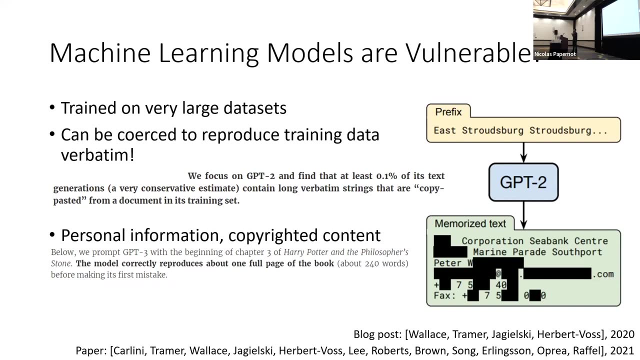 models can be trained privately in a surprisingly simple way. just recall, you know there's a slide I had earlier. we're gonna. you can try to think of a common use case as trying to prevent, uh, outputting parts of the training data verbatim as an example. uh, the idea is we want some sort of machine learning model we can put out into the. 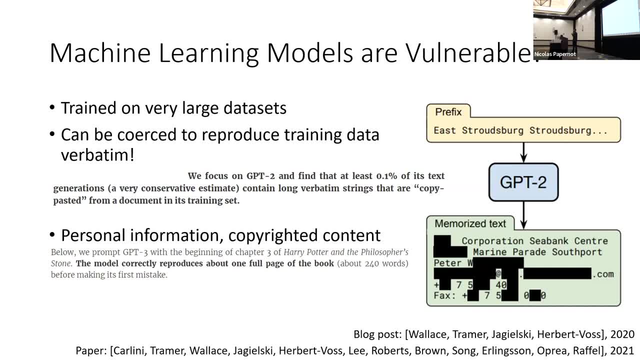 wild where anyone in the world can look at it and no matter what they ask if it, even if they look at the weights, maybe they- uh, you know- ask it all sorts of weird queries. nonetheless, it shouldn't be able to violate the privacy of the training data set in the way, uh, that we care about, for 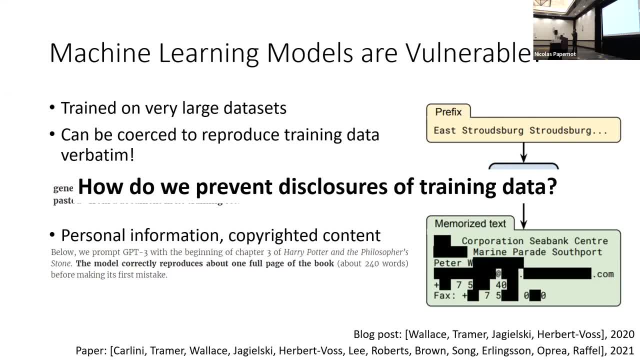 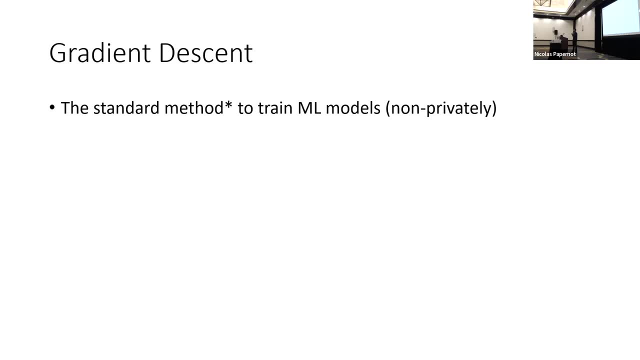 example, amongst other things that shouldn't violate. it should prevent against disclosures and just leaking uh data points verbatim, and you know, let's build our way up on how to do this. well, suppose we didn't care about privacy. what we would do is just use gradient descent, which is the standard method to train ML models. 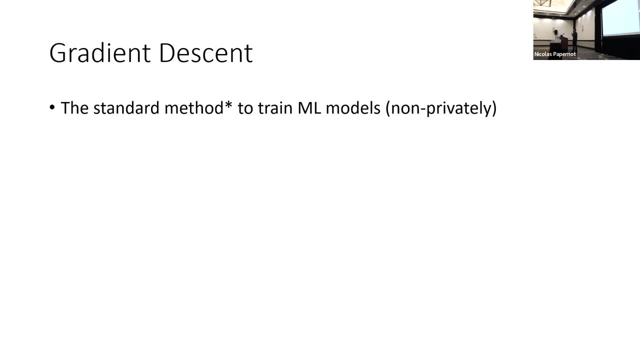 you might be thinking that, okay, maybe stochastic gradient descent is what maybe people might use. put a pin in that we'll return to it. let's focus on gradient descent first and I don't think I need to tell maybe anyone in this room what gradient descent is essentially: have some data, set what. 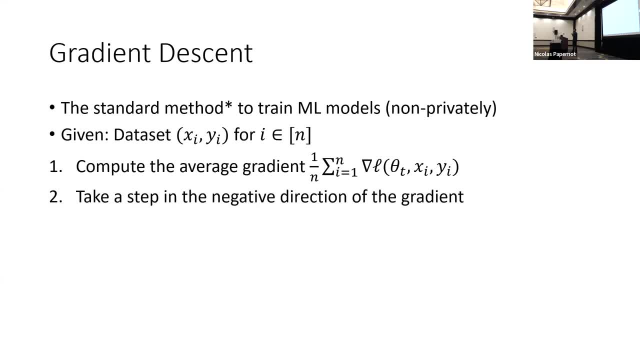 you do is you compute the average gradient, take a negative step, a step in the negative direction of gradient, repeat. so this is gradient descent, non-privately, hopefully, familiar to most people here. the nice thing is we'll say: just see just a few tweaks to this procedure, two very simple and 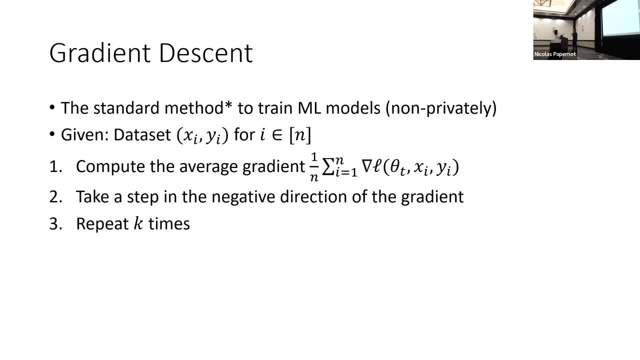 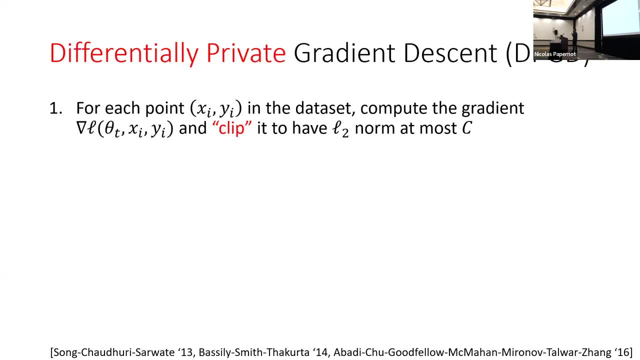 intuitive tweaks will make it into something which is differentially private. so the the differentially private gradient, descent, or dpgd, is the following: what we're going to do is we're going to start again by computing the gradient of every point in the data set, but then we're going 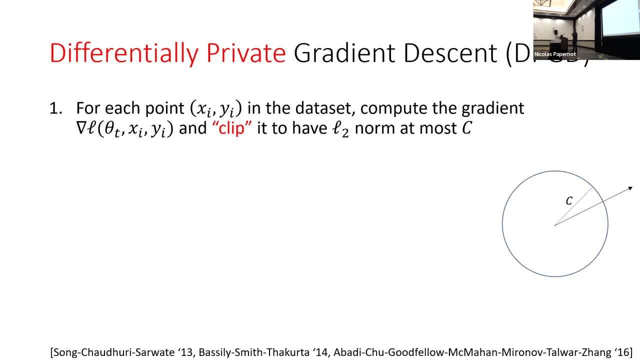 to do a clipping operation to make sure the L2 norm of the points is bounded. so to give you an illustration of what that looks like you can see here, suppose this black arrow here is our gradient for some data point. but what we're going to do is we're going to essentially clip it or project it. 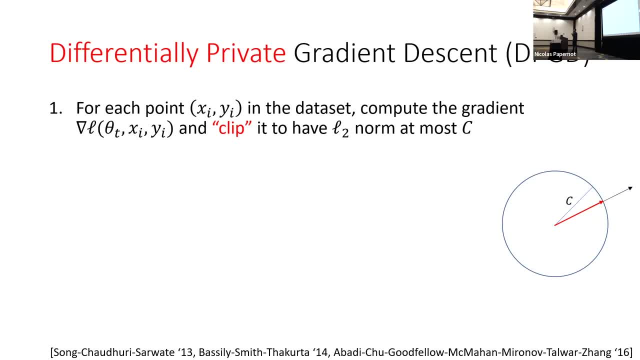 to this ball of L2 radius. essentially, just if any gradient is too big in magnitude, clip it, shrink it down to this ball and, intuitively, going back to the principle I mentioned before about the sensitivity being an important feature- if you didn't have clipped gradients, the sensitivity of an average could be unbounded. you could have an incredibly large gradient which 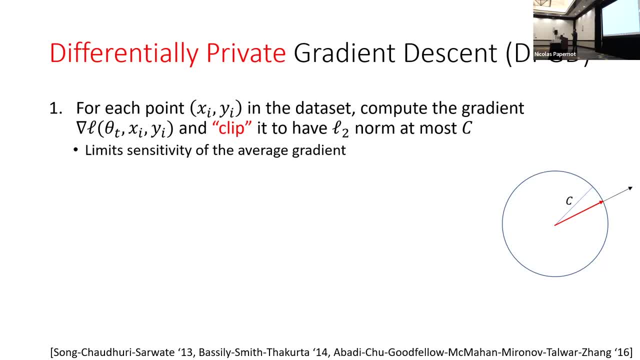 would just totally violate privacy of one individual point, potentially. so what we're going to do is we're going to clip, essentially to limit the sensitivity of the average gradient. so once we've done this, then we do as before: we average the gradients. but then the last step: 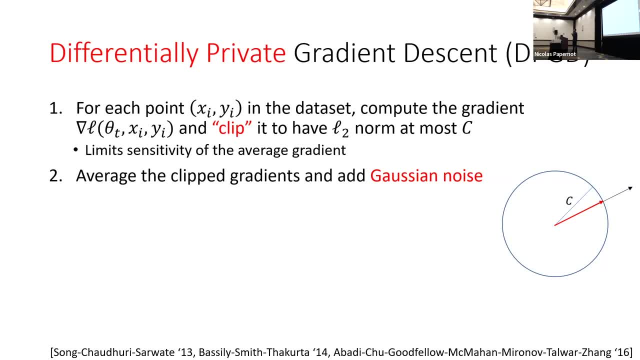 which comes in for introducing privacy is we add Gaussian noise to the average gradient. the other two steps are the exact same. you take a step, repeat K times for some large value K. but so I just want to emphasize the two differences between gradient descent and private gradient. 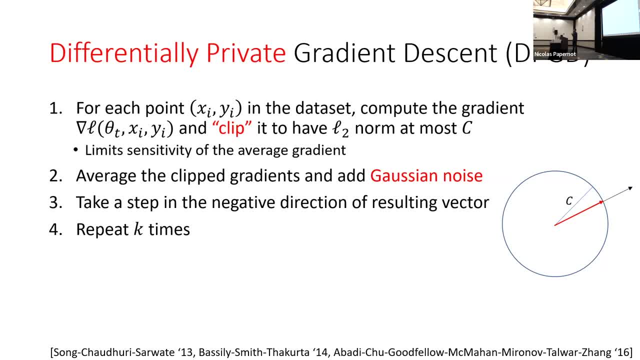 descent are. you clip the individual gradients and then you add Gaussian noise. that's it, very, very simple and intuitive in my mind. uh, changes. now you might be wondering: why is this private? why? why is this at all a reasonable thing to do? well, I claim that this is exactly. 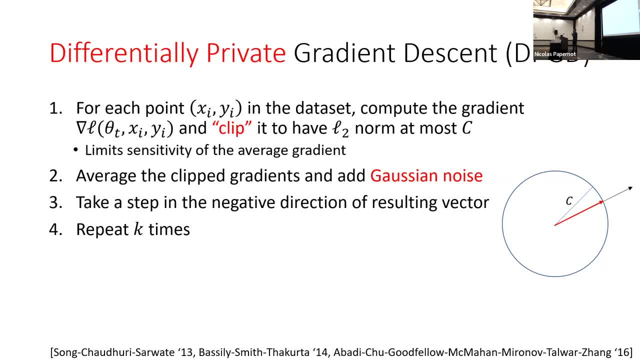 the things I've told you already. in particular, if you look at steps one, two, addition of Gaussian noise to a function with bounded sensitivity is exactly the Gaussian mechanism which I told you before adding Gaussian noise. and okay, that's one step, but in fact, since you repeat it K times, it's. 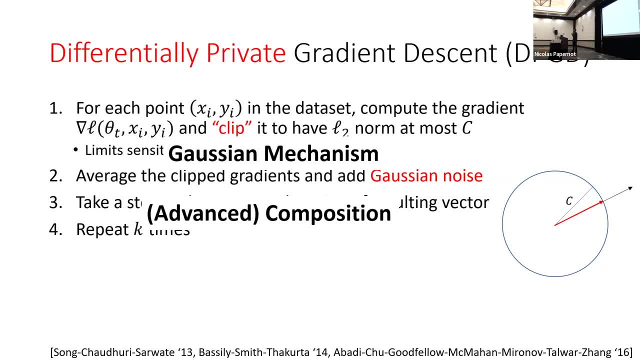 essentially doing the Gaussian mechanism, K times and therefore we're going to use advanced composition to argue that releasing all K of these iterates is also going to be differentially private, just using advanced composition. so that's it like really. this is how you train a machine learning model privately. you do the Gaussian mechanism, a. 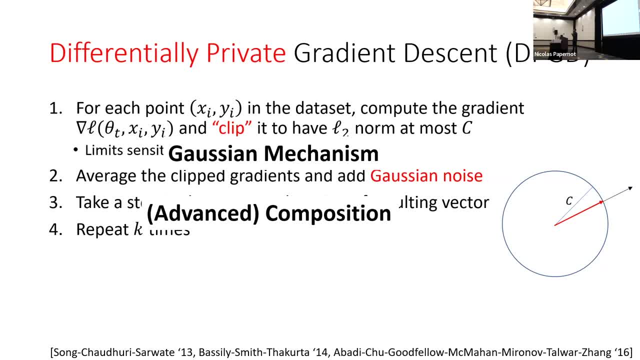 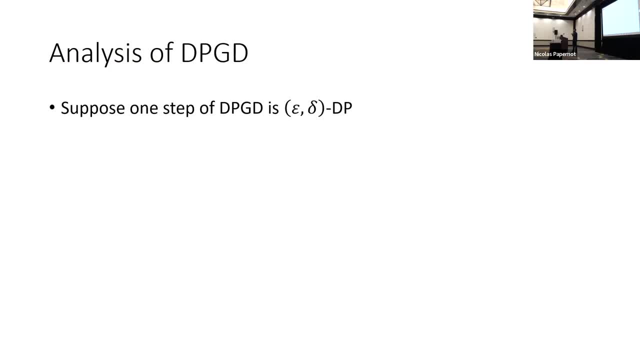 bunch of times and and it works. um, yeah, and and the analysis. you know I'm not going to be labor this too much, but it's very, very simple. suppose you know you set the parameters right for how much noise you add, uh, and such that one step of dpgd is going to be Epsilon Delta differentially. 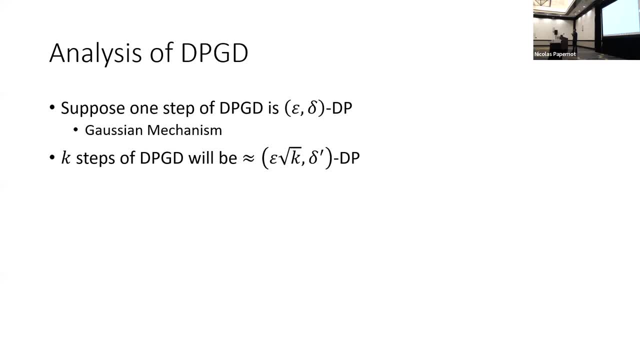 private. well then, you know K steps. just using this advanced composition theorem, uh, will give you that. the overall privacy disclosure is on root K and Delta Prime for some. I'm not going to get into what Delta Prime is, but essentially just use it. advanced composition, and that's the simplest way to do. uh analysis of private gradient. 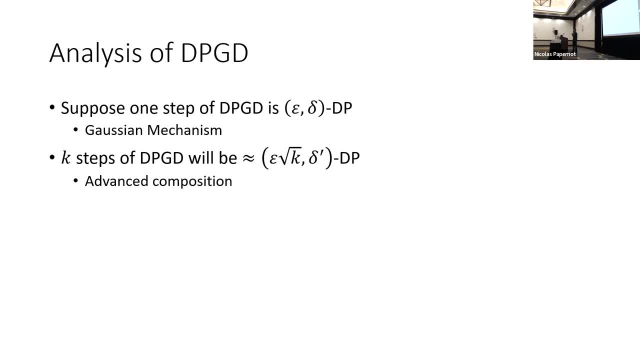 descent, that's it. like you, you know everything right now to train a machine learning model with differential privacy, a very, very simple change to, uh, the standard procedure? um, it's not going to be. there's not the best way to do it in the sense that you need to do better accounting, like there's. 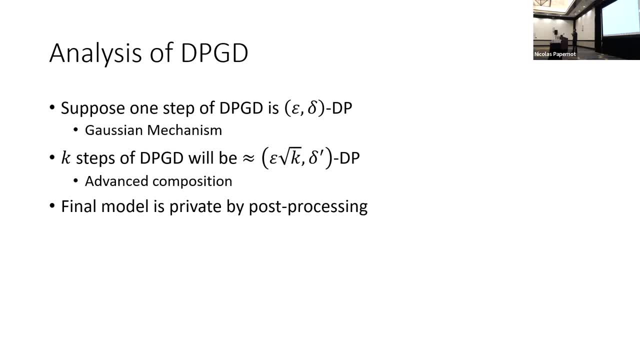 additional tricks you can do like one. one thing I'll mention, oh sorry, yeah, an important thing is the fact that, uh, the final model is going to be private by post-processing, in the sense that you know, I tell you that the iterates and gradient descent are going to be. 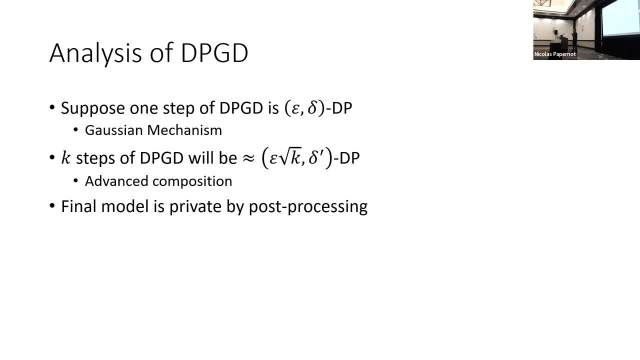 private, but in particular, a function you do with this- uh, these iterates- is basically just release the final model and after that I can give this out to anyone in the world and by post-processing they won't be able to violate the privacy of the training data set. so the downside of this method 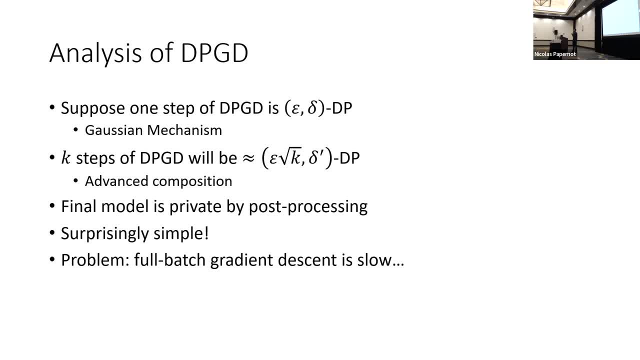 is that nobody in practice for very large problems might use full batch gradient descent. they might use a stochastic gradient descent and the fortunate thing is it's very easy to adapt it to that. I just want to start with a simple case. you can see really just the Gaussian mechanism, but stochastic. 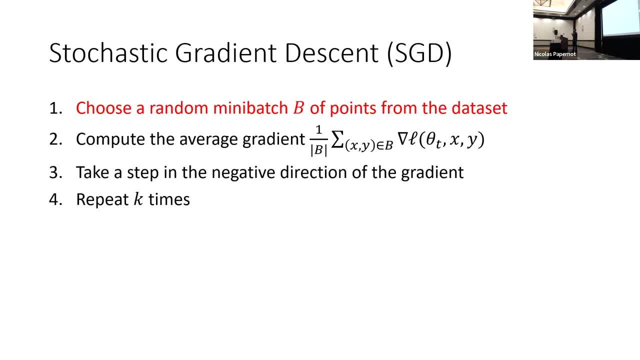 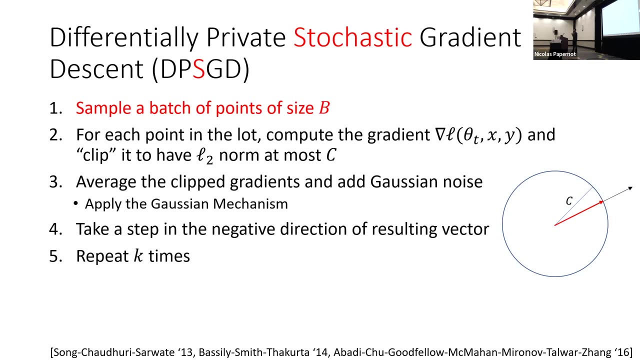 gradient descent is almost the same thing. the one difference is that you do some random mini batches, or, you know, ordered mini batches from the data set, and then you average over each of these many batches and repeat, and it's very easy to uh, just basically plug this into dpgd and it becomes dpsgd now, where the first step is just randomly sampling a. 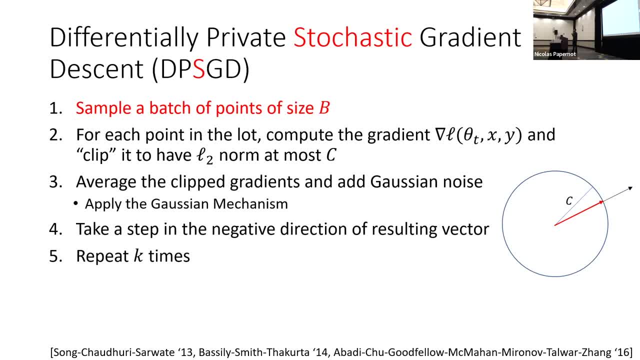 batch of points of whatever size. I'll comment that there's a, like I said, uh, before I gave you a simple analysis, but there are better analyses you can do, in particular the, the. I'm not going to get into this technically, but there's an intuitive fact that, okay, we're just randomly sampling a set of 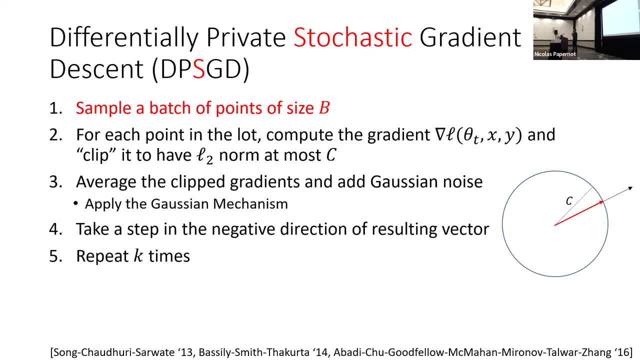 points, suppose their over overall data set is a million points, but we just sub sample a mini batch of size, say, uh, 64, 128.. well, intuitively, that should give us some better privacy, right? because we're not even looking at the whole data set for that query. so the property known as privacy amplification by 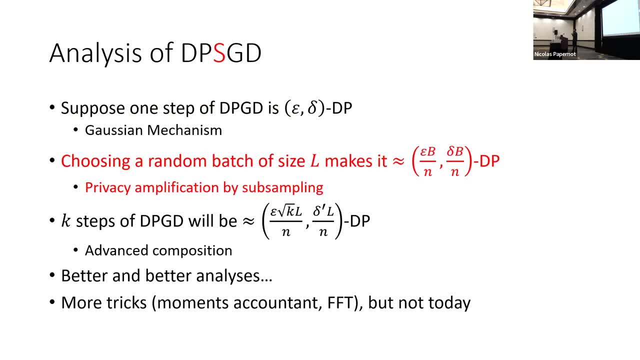 sampling, a privacy amplification by sub sampling which improves- sorry, that should be a- B- which improves the privacy, just based on the fact that we're only looking at a subset of the data. so if you didn't follow that, don't worry, but the main thing is that 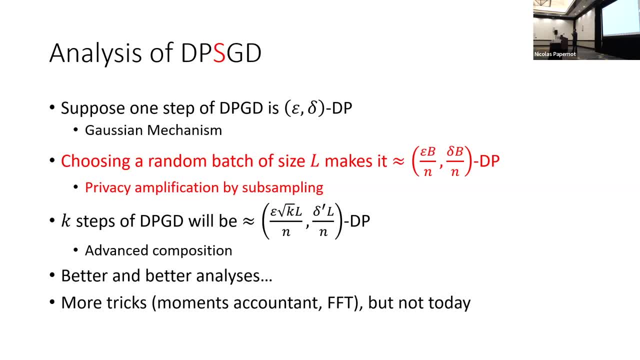 like. I introduced another new thing which is used to uh analyze privacy in this type of setting. and then there's more tricks you can do as well, things like what are known as moments accountants. there's fast Fourier, transform uh methods to do privacy accounting, but if, if you're more careful. 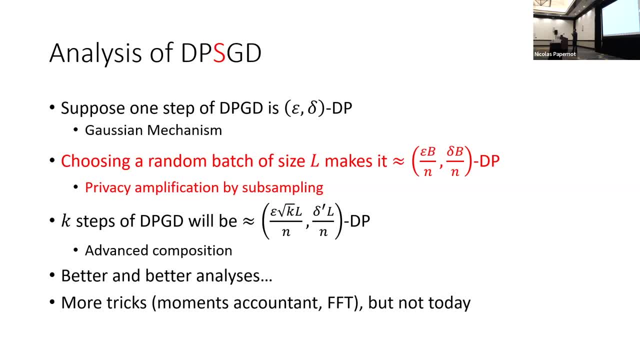 and clever with the math, then you can basically give a better private analysis of the exact same algorithm, and this might sound complicated, but the good thing is that you know all these analyses and And you know implementation details, which are kind of tricky. you have to work through them, they're tough, but you don't have to do any of that work. 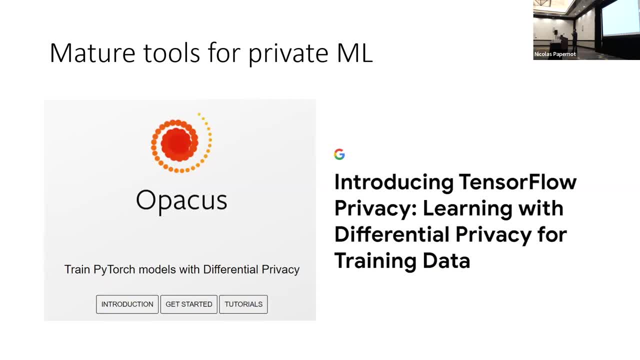 The good thing is that there's very mature tools at this point. you know, the same wouldn't be true, say, 10 years ago, but now there's a Opicus and TensorFlow, privacy, which are very mature and useful tools where you can train a model privately. 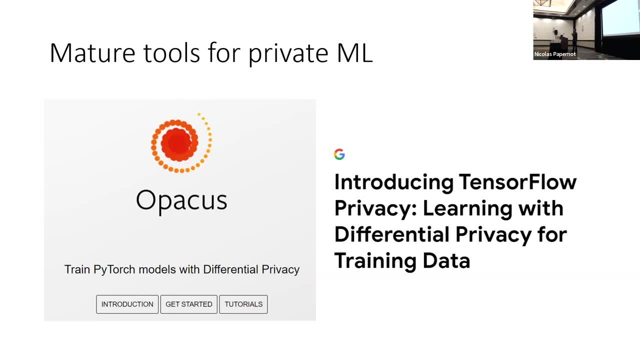 And you know, if anyone here is interested like you, can basically go back to your computer and probably, if you are comfortable training machine learning models, within like less than an hour you can get a private machine learning models trained on some basic MNIST cases. it's not that hard. 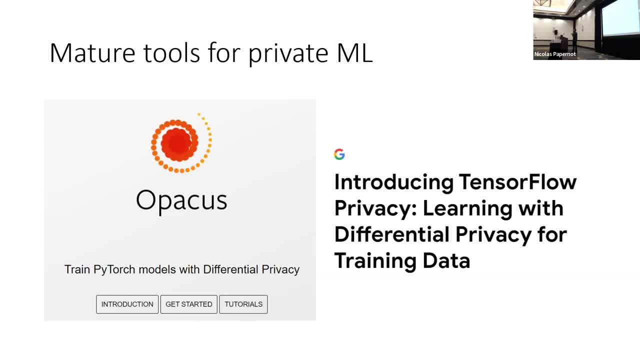 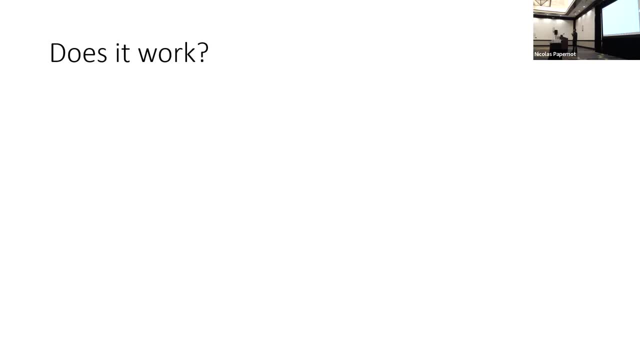 These are very nice, with great tutorials available. So now the big question is: does this really work? You know, I've told you how to train a model privately. it's going to be private, but is it any good? And yeah, let's see, I'll just go over. 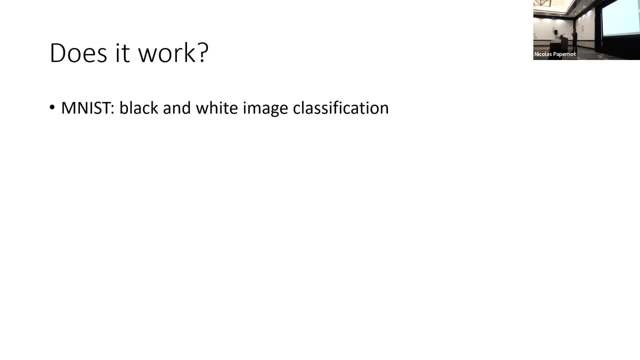 To basically conclude a few simple cases and show you what is known in terms of private machine learning on some classic benchmarks. a natural place to start for any question is MNIST. non-privately you can get effectively 100% accuracy on MNIST- you know close enough. and privately you can get, with pretty reasonable privacy parameters, 98 or 99% accuracy. 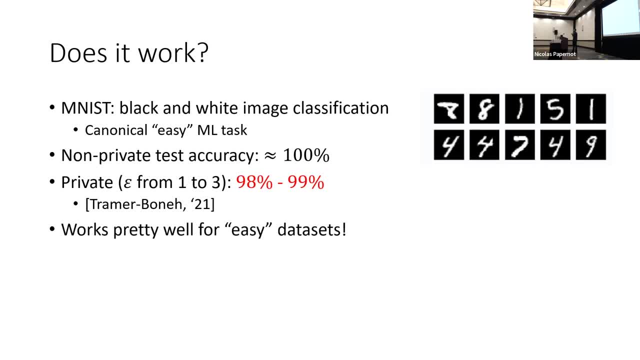 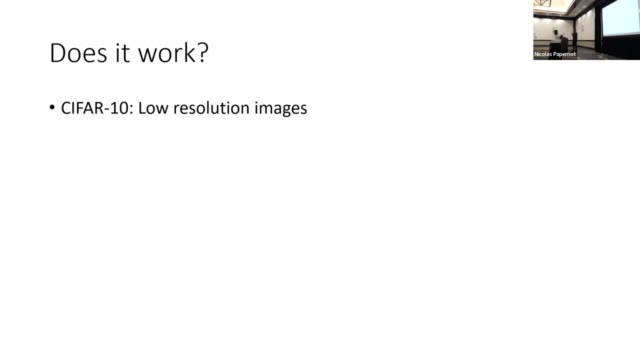 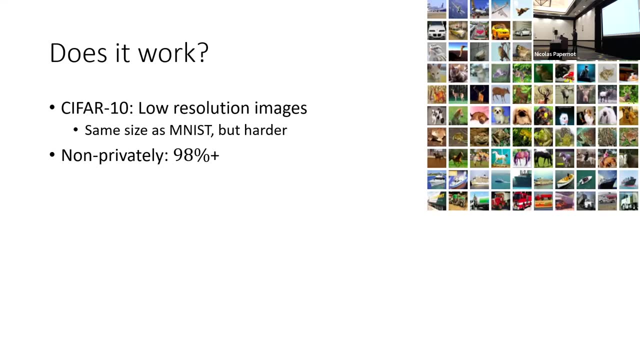 So it seems like differentially private machine learning is pretty good for, say, MNIST. It gets a lot harder, even for the next data set, to be honest, CIFAR-10, which you know, most people here I think are familiar with. but non-privately you can get, say, 98% accuracy, but privately the state of the art is kind of a lot worse. you know, with various different privacy parameters there's different things you can get. but even in the best case, with epsilon equals eight, you'll see that the error jumps from, say, 2% to almost 18%. 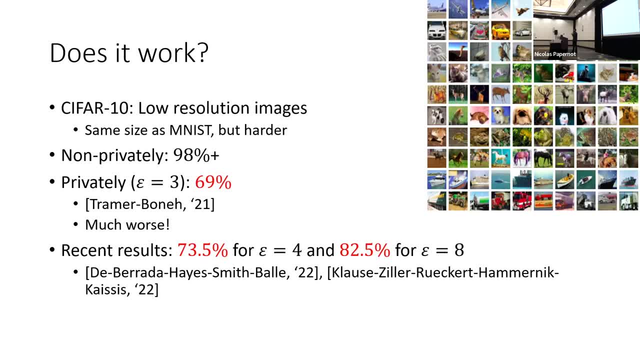 So this is, you know, much worse than what you would get without privacy, and this is kind of. people put a lot of work into trying to improve this. I think these results are actually very nice that they're able to do so well, because it's not an easy problem and in some sense, one of the faults for this is because CIFAR-10 is a relatively small data set for the complexity of the task that we're doing. 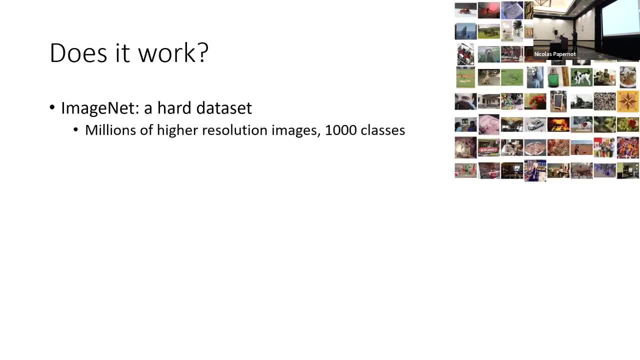 And you know, for harder tasks like ImageNet, you know all bets are off non-privately. maybe you can get like 87% top one accuracy, but privately even with epsilon eight, you know, the state of the art is 32% accuracy and even this was very difficult to achieve Like. I think this is very impressive that we were able to even able to get that. 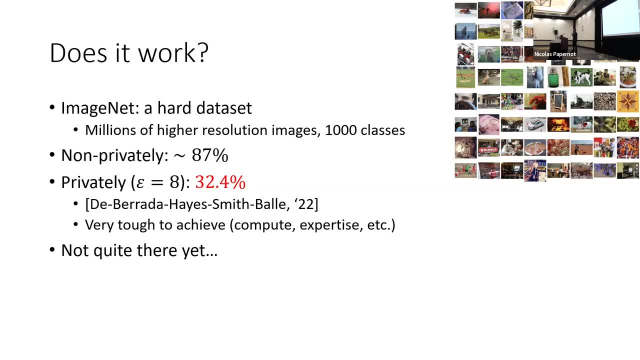 So the kind of takeaway from this is that if you want to do private machine learning for complicated tasks, it can be. it can be kind of challenging, Yeah, and it's still far behind non-private machine learning. There's a lot of stuff to do. 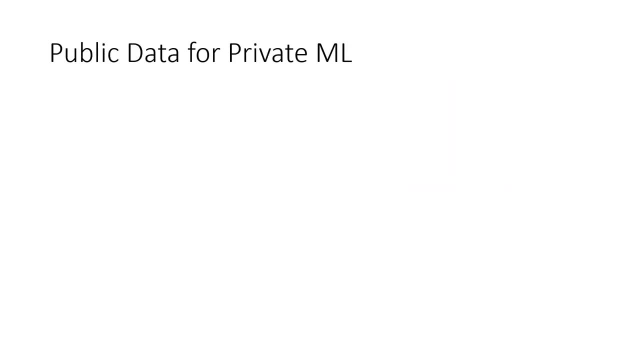 I'll mention in the very last part of this that you know, one recent trend which I've been interested in, others have been interested in, which can alleviate a lot of these issues, is using public data for private machine learning, which is kind of a common trend even in the non-private setting in the sense pre-training. 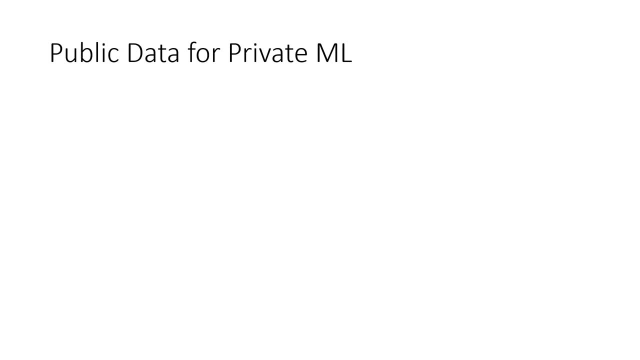 and fine-tuning the common paradigm now in, uh, in the non-private setting, and that lends itself very nicely to differential privacy. the intuition is: maybe first you can pre-train a model with, uh say, public data, uh say, just downloading images from the internet, uh say, google image search. 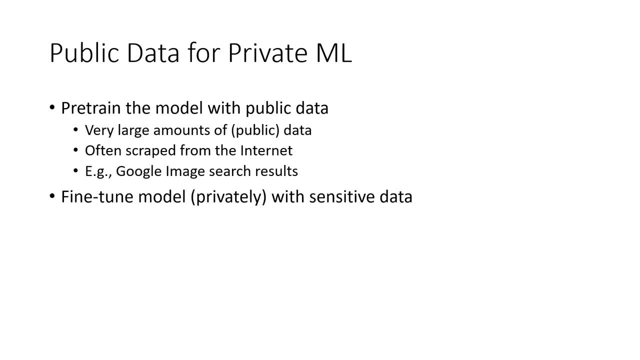 results and then after that, once you've done something like that, you can fine-tune the model privately using dpsgd with uh sensitive data. and for example, imagine you want to do chest x-ray classification- this might be privacy sensitive. uh yeah, and you would train this with dpsgd. so you 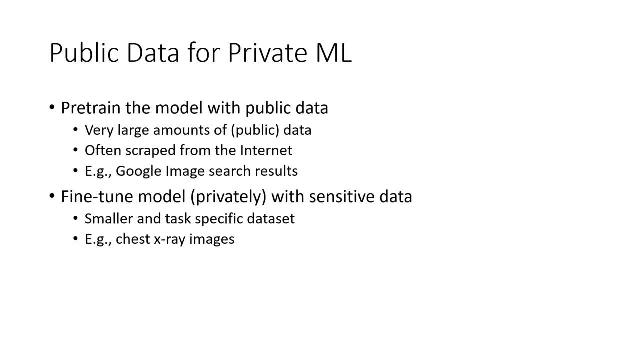 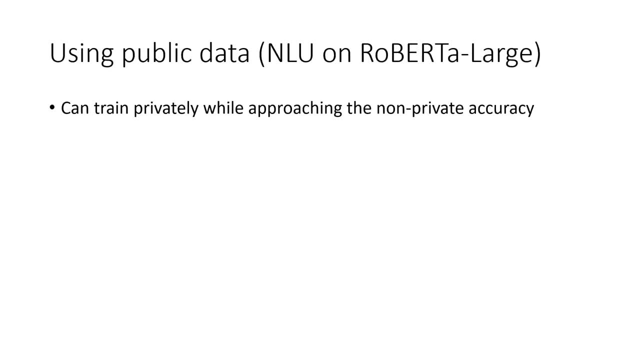 can see how i'm kind of delineating the data set into one data set which is public and there's no privacy considerations. it's either normal, but then fine-tune with privacy and this helps a lot. um, we have some works on language models which i'm not going to mention, but the utility is very good. 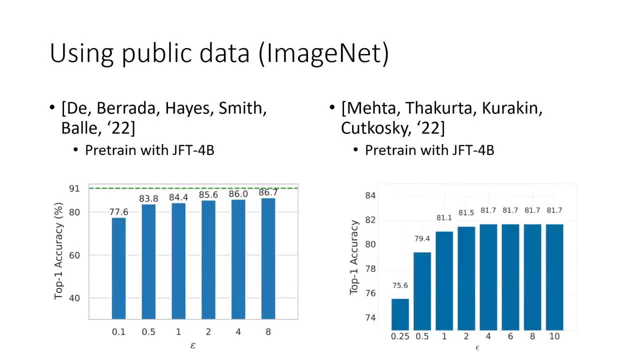 but i'm going to tell you about some recent works, uh, on image net, which you can see here, with even very small privacy budgets, uh, then you still get very high accuracy compared to the state of the art which is, i guess- i don't know either- 87, 91 somewhere around there, but the point is it's very close to 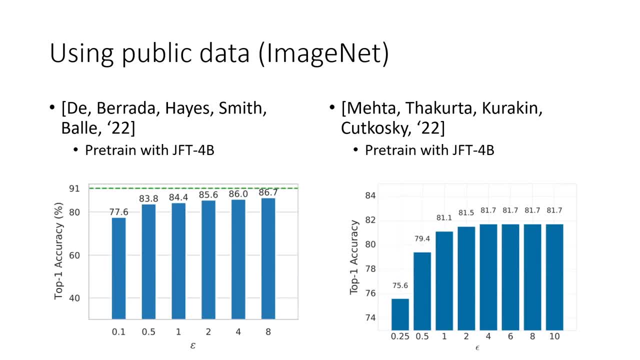 uh, the non-private state of the art, uh, that you can get. so, essentially, it seems that public data can alleviate many of the problems with private machine learning's utility, and so i think it's a good point to make, and if you look at the data set in the data set, um, it's an interesting direction. 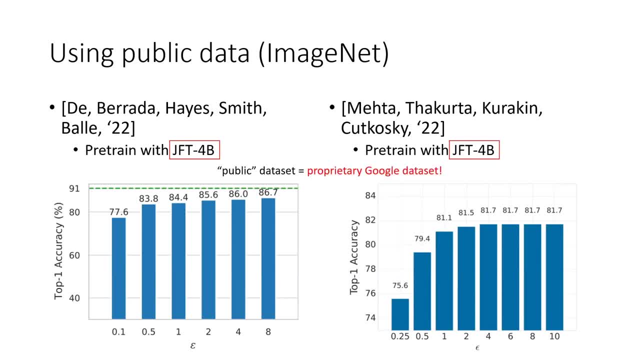 to move forward. there's a few caveats here, including, for example, if you know what jft4b is. this is not a public data set, it's a proprietary google data set, um. so there's some, there's some critiques which uh myself, florian and uh nicholas carlini have, um, but i'm not going. 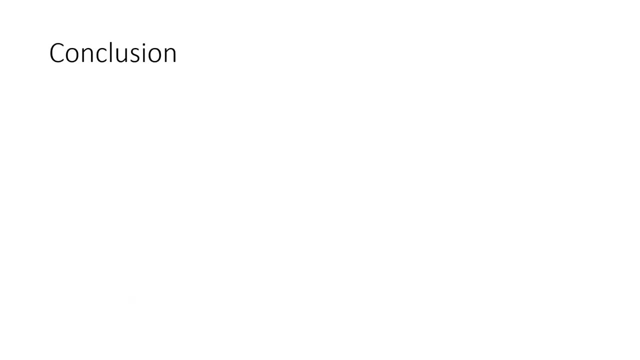 to get into that today, but yeah, i think there's an interesting direction to moving forward. but in conclusion, uh, i just want to wrap up and say differential privacy is a strong and useful you about a bunch of fundamental tools and building blocks and a bunch of convenient. 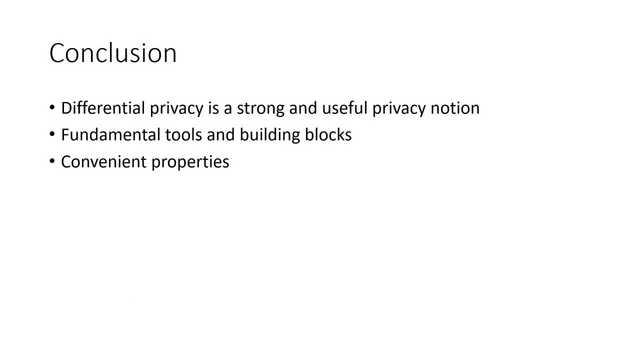 properties which make it possible to build convenient, uh, to build much more complex systems out of these, in particular how to do private machine learning, which you know, just just giving gaussian noise addition and repeating that many times. it's shocking to me that something can actually like that can actually give real models which are private and so effectively.